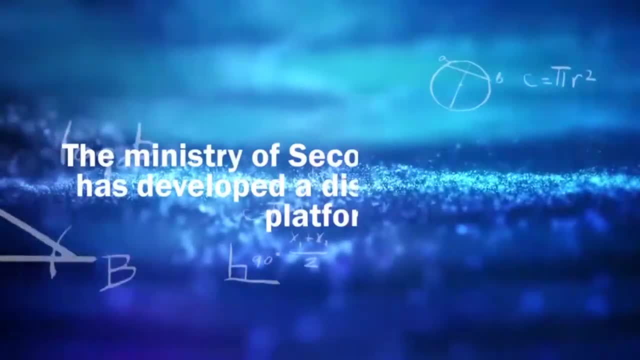 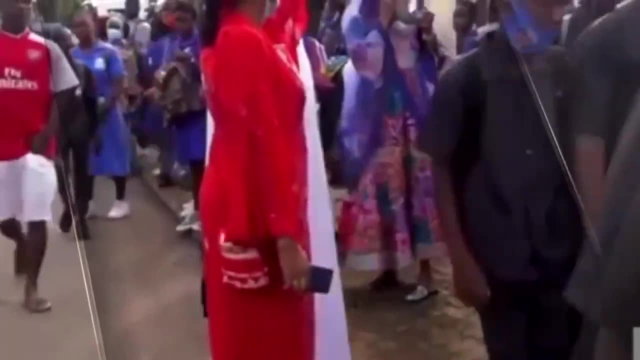 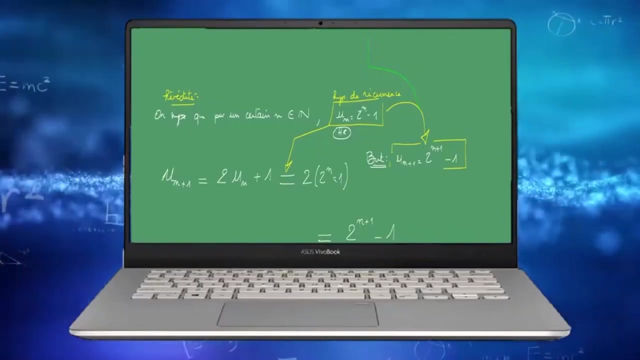 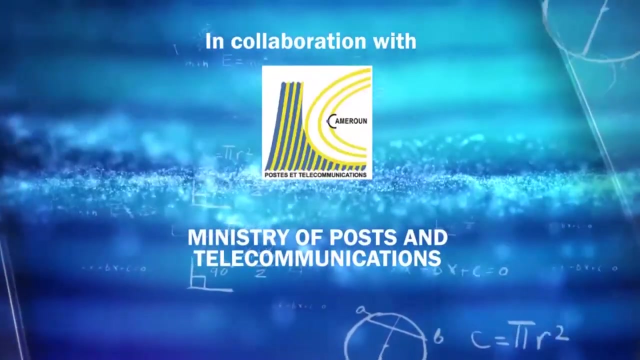 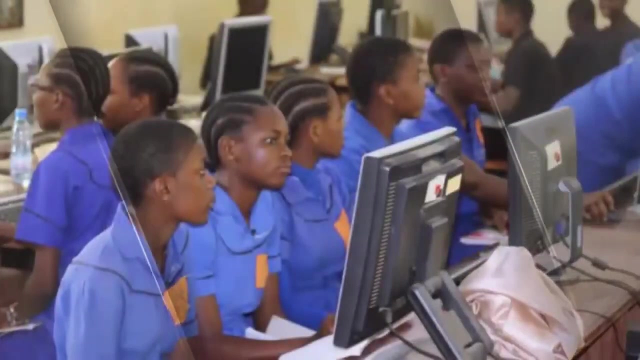 The Ministry of Secondary Education has developed a distance learning platform for students of secondary education in Cameroon: A series of lessons taught by qualified teachers for secondary school students, Under the stewardship of Professor Pauline Nalovalyonga. in collaboration with the Ministry of Posts and Telecommunications, Camtel, CRTV and UNESCO, We are introducing 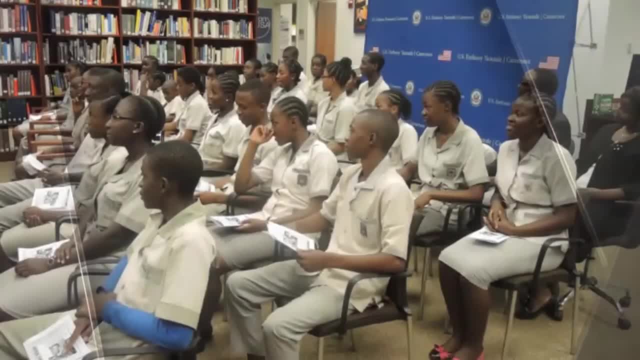 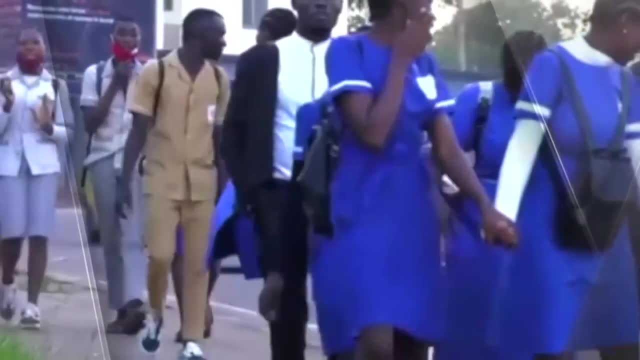 distance learning as another teaching and learning method which is different from the traditional classroom setting that you are all used to. In the distance education mode, you are not with the teacher in person, so take your time, relax, listen to the teacher. 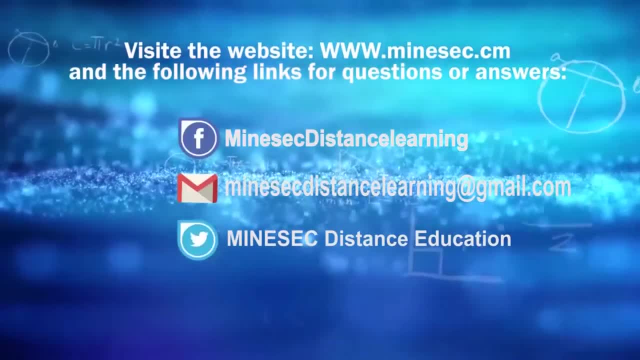 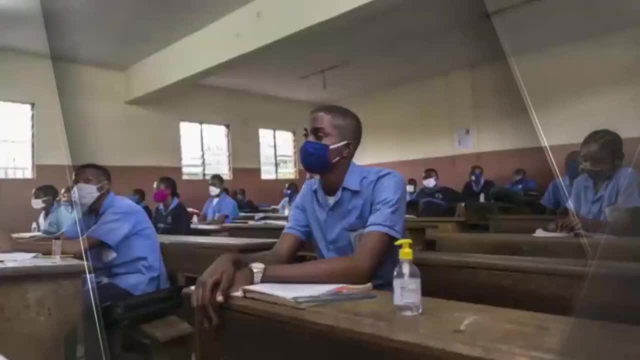 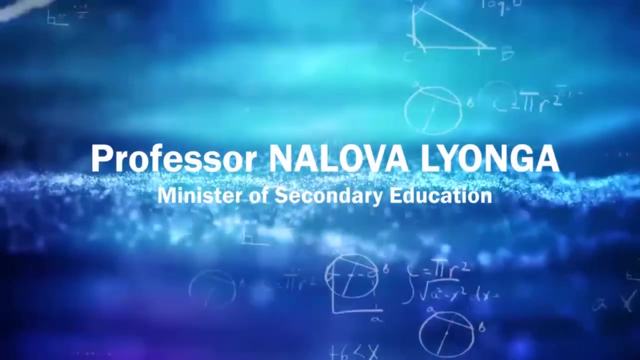 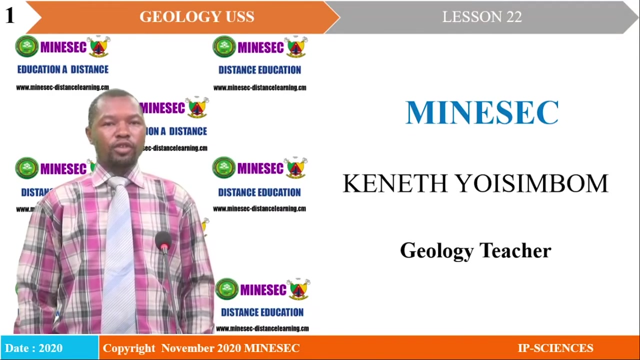 take down notes and visit the following links for any questions or answers to your questions. Take it in your stride. This is Cameroon's solution to COVID-19 and beyond. Professor Nalovalyonga, Minister of Secondary Education, Welcome to lesson 22 of your distance learning session for geology, opacite science with 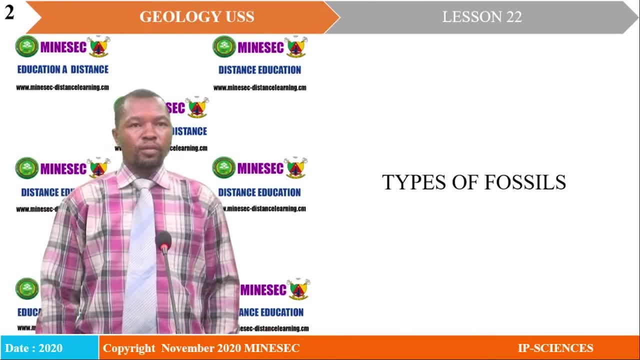 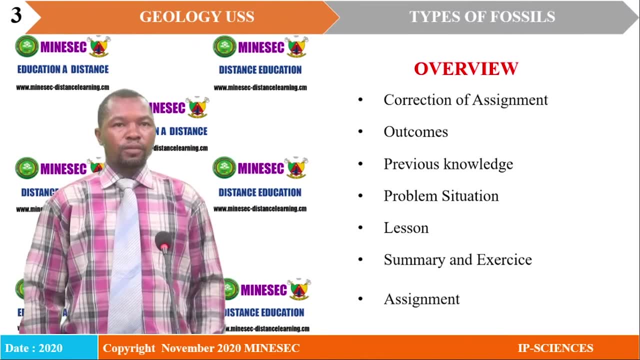 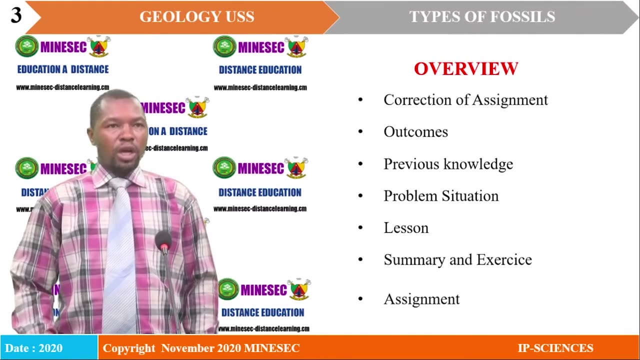 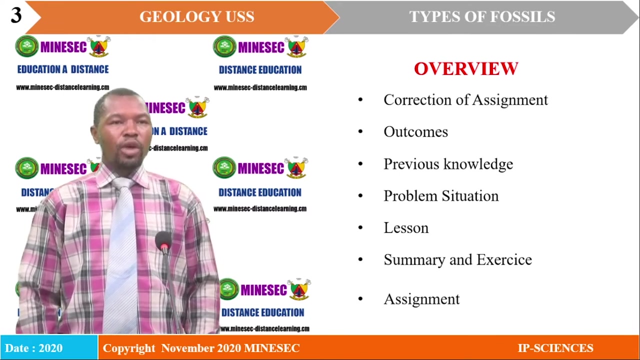 Kenneth Yosimbom. Our lesson 22 is titled Types of Fossils. The lesson overview includes correction of assignments, outcomes, previous knowledge, problem situation, the lesson summary, exercises and we shall end with an assignment to take home. 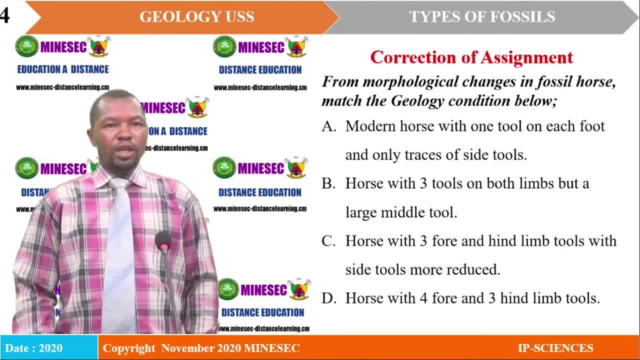 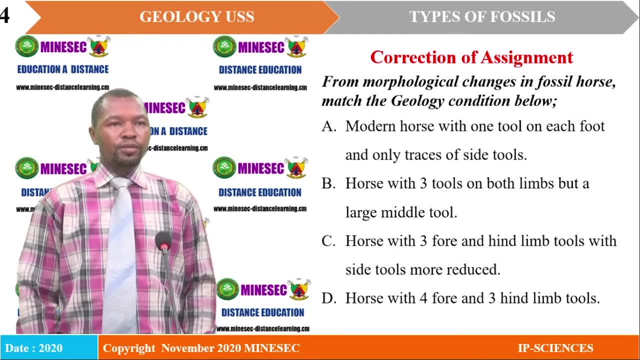 Correction of assignment. During our last class we had some work to do at home. We are required to look at the analysis, the morphological changes in fossil horse, as well as the geological conditions, and to relate them with their geologic appearance within the time scale. 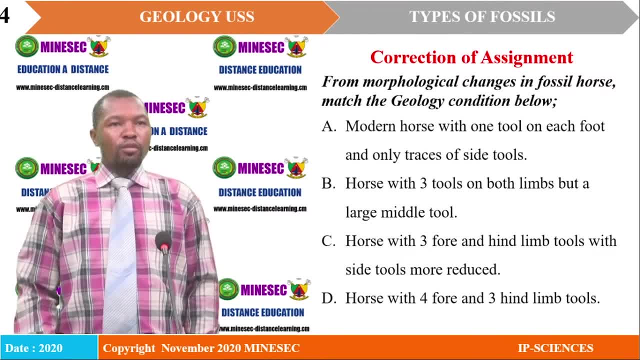 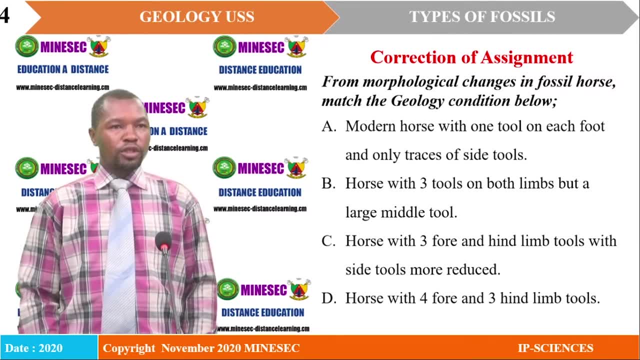 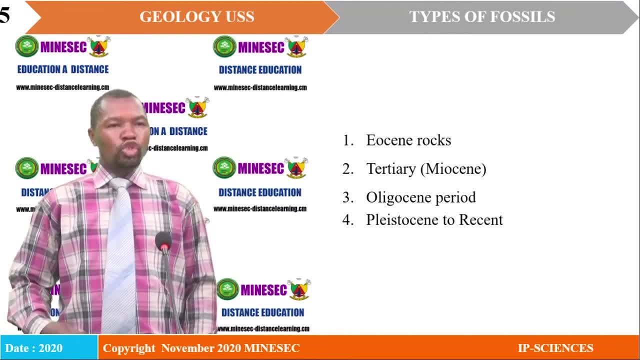 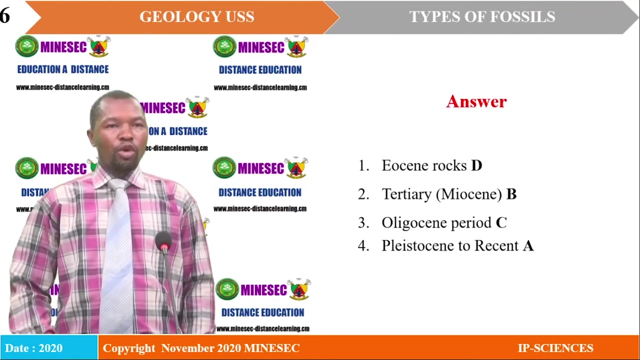 looked at the different morphological features. we are now going to relate to the geologic time. that was the nature of the assignment. if you approach this assignment correctly, then you are going to have that. the Aocene rock will relate to D, that is, in the day or scene. the horse had four, four and three high. 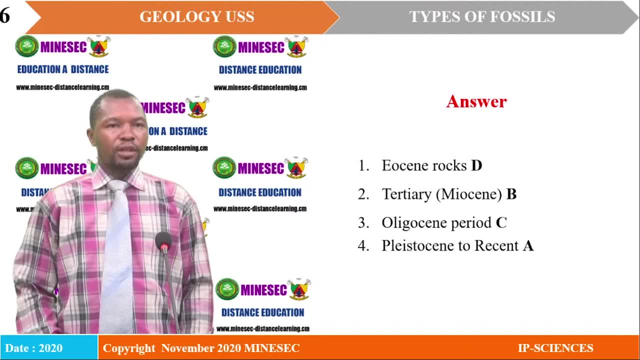 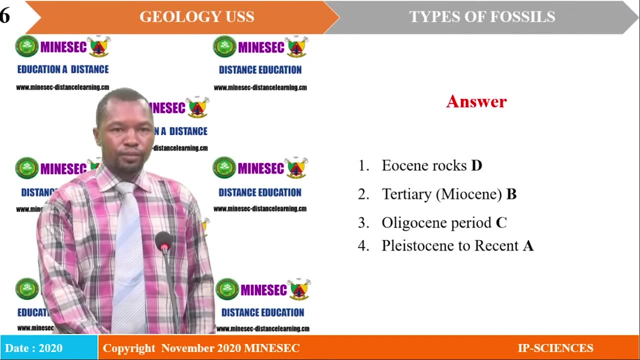 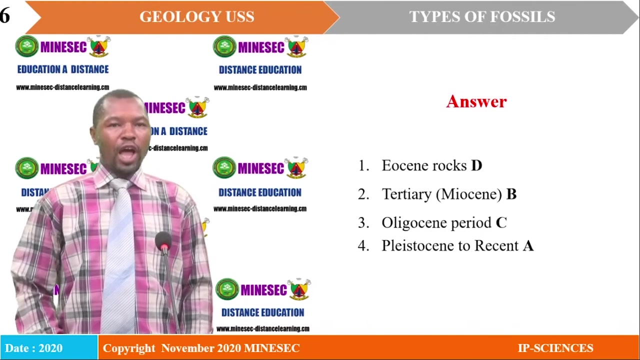 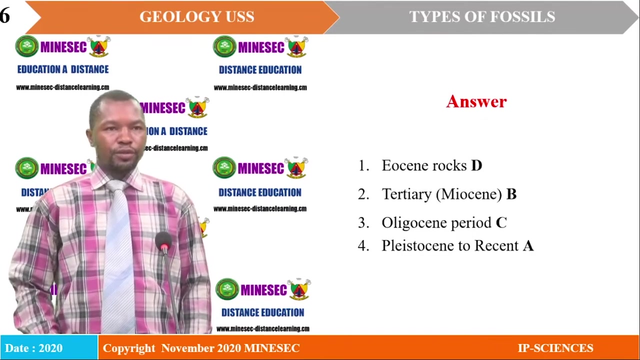 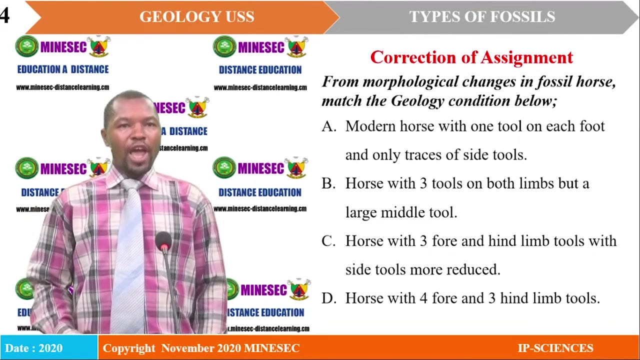 limb tools. then the tertiary horse, hadeast letter to B, that is the horse with three, four and high limbs. then Then the Oligocene period had the horse with three, four and hind limbs, limb tools with side tools more reduced. Then the last case related to A. that is the condition where the condition that we can 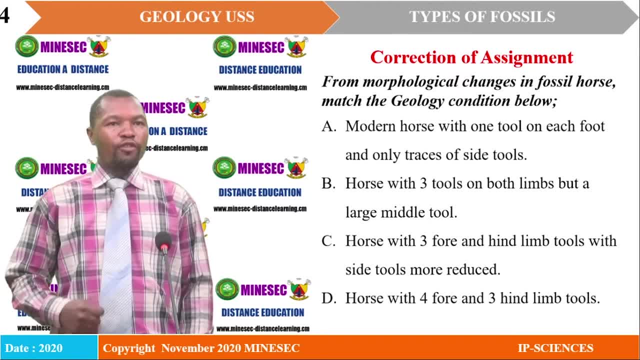 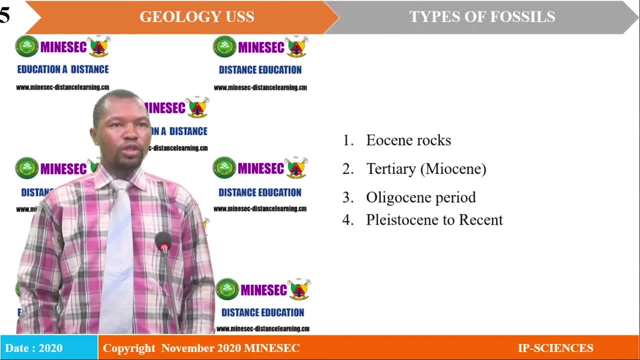 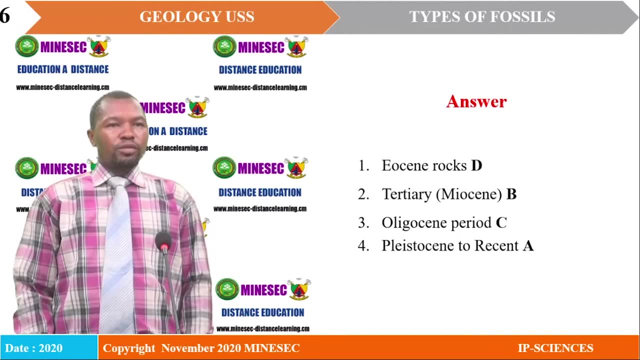 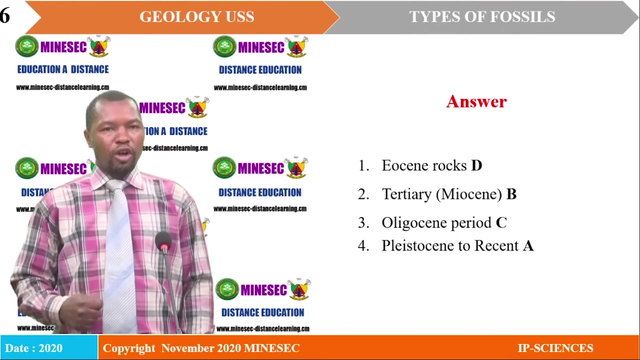 refer to as the modern horse with one tool on each foot and only traces of side tools. That was the right approach to that assignment. Now, it was equally to help us to understand the evolution of the fossil horse, as well as give us a pattern on how evolution works. 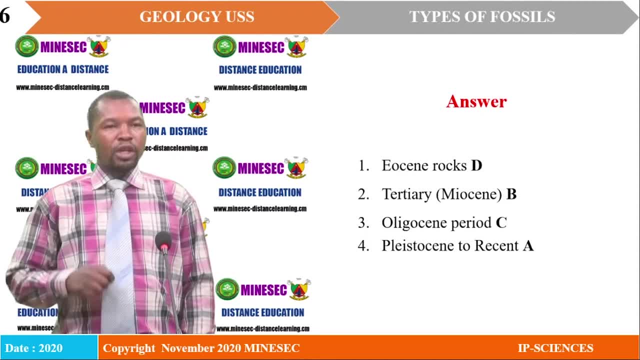 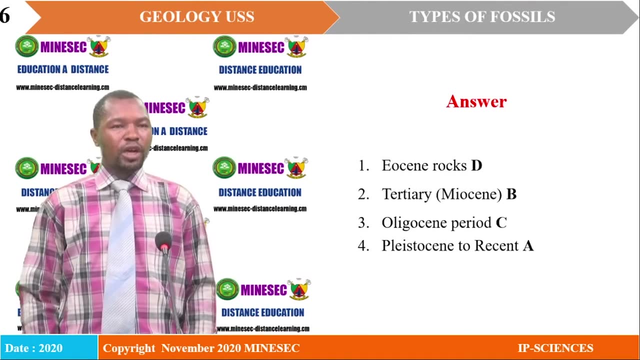 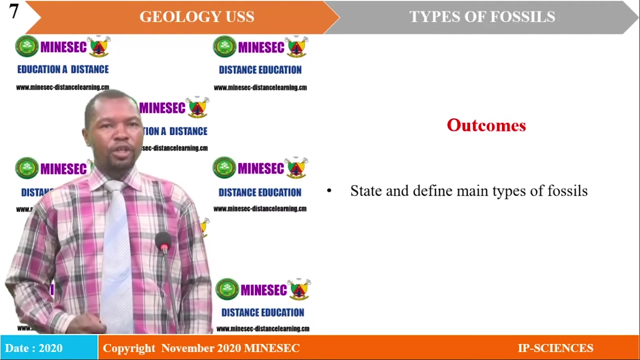 The evolution in the different fossil groups happened Like. we already established that as rocks become younger, the fossils become more complex. That was one objective that we were supposed to attain in the course of doing our assignment. Now, the outcomes of our lesson today, which is titled Types of Fossils, include that at 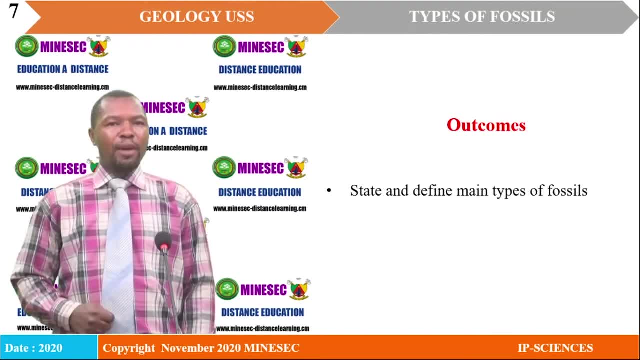 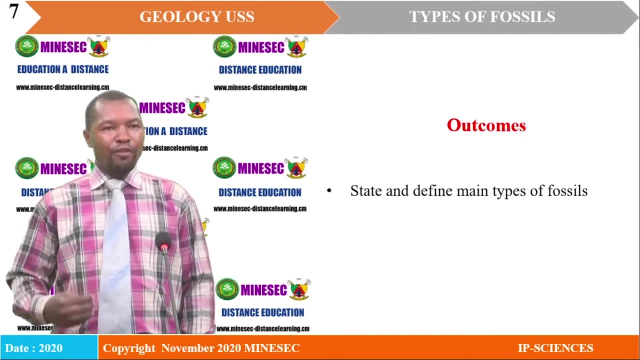 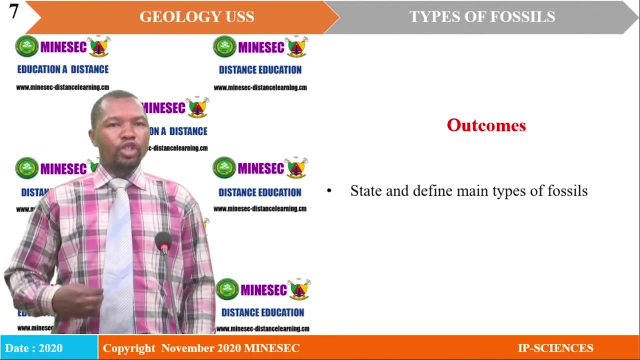 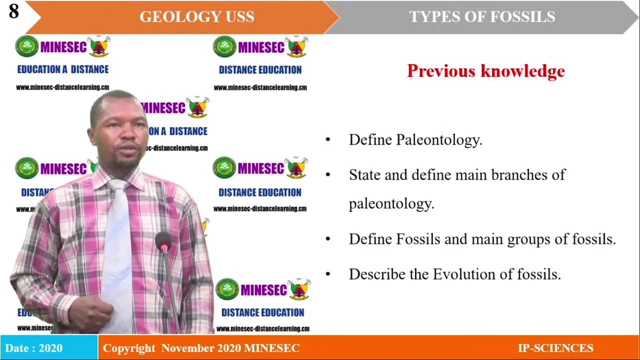 the end of this lesson, You shall be able to state and define main types of fossils. This lesson we will have it in parts, meaning that because there are many types of fossils, we are going to have it in different lessons before we can unravel the main types of fossils. 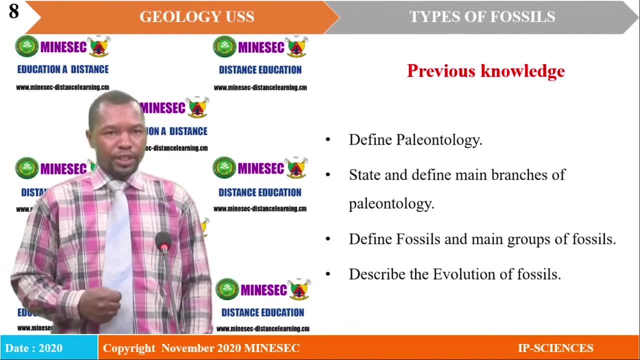 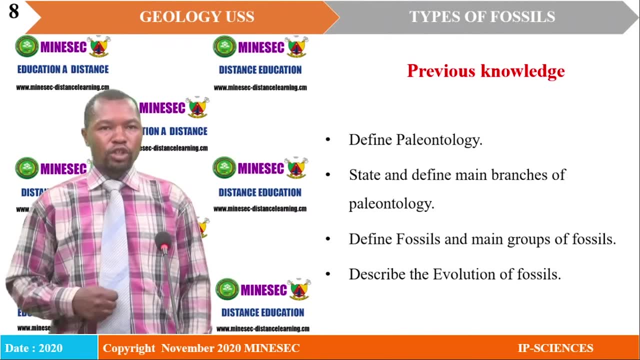 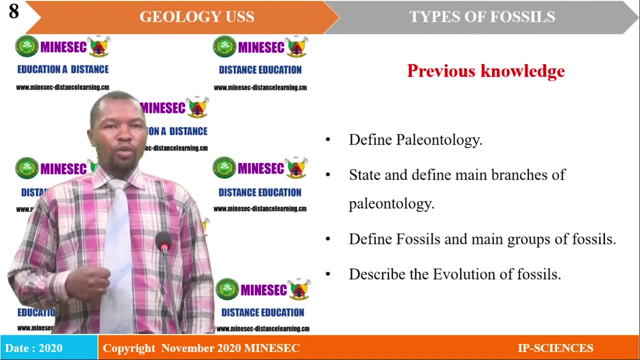 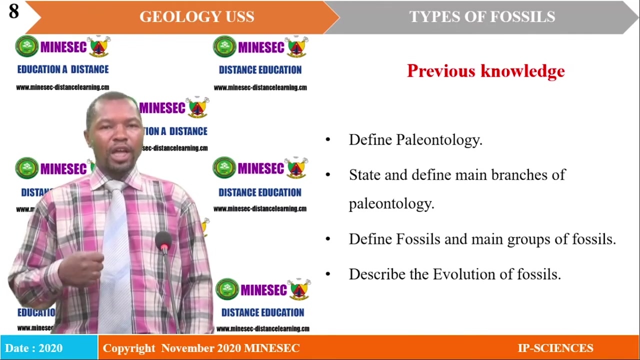 Previously, we had studied on the scope of polygons. This lesson is about polyontology. So we can now define polyontology. We can now state and define the main branches of polyontology. We can also define fossils and main groups of fossils. 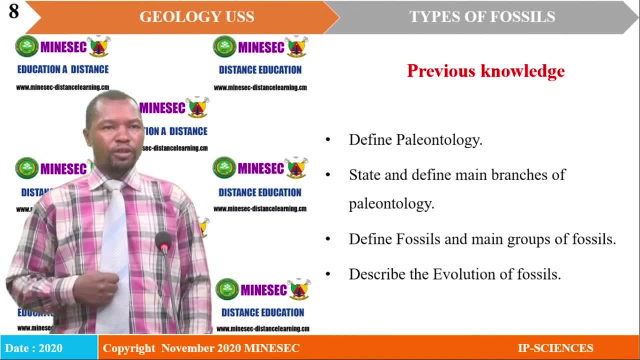 As well as we can be able to describe the evolution of fossils. This knowledge that we had during our first lesson is going to help us understand well the evolution of fossils and the evolution of fossils. That is what we are going to be doing today. 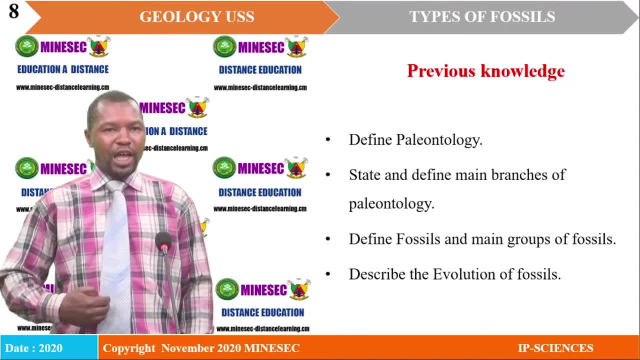 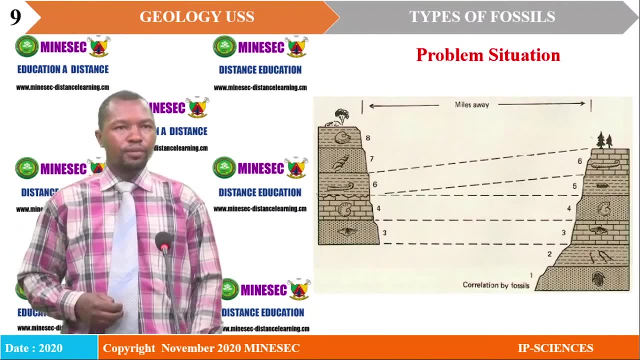 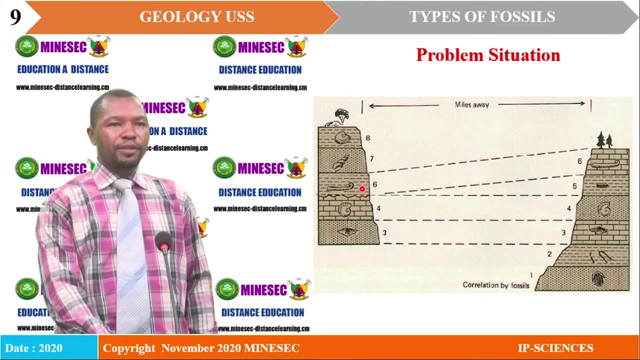 Thank you for your attention. Thank you different types of fossils, as well as be able to reallocate them into the different branches of paleontology. now our problem situation. you observe there's two blocks. again, those are rock sections. all of them are layered, but what is peculiar is the fact that each of the layers have a particular fossil. 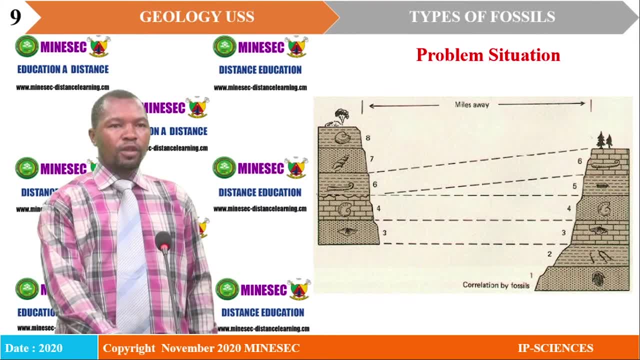 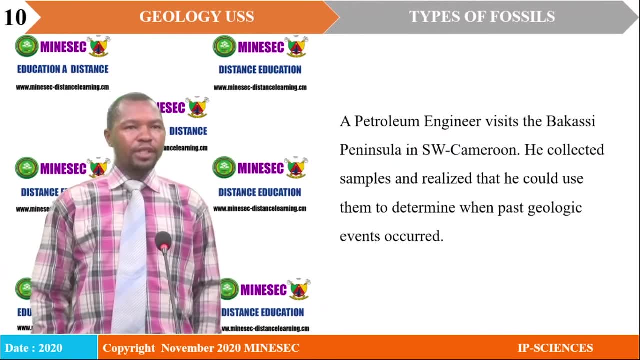 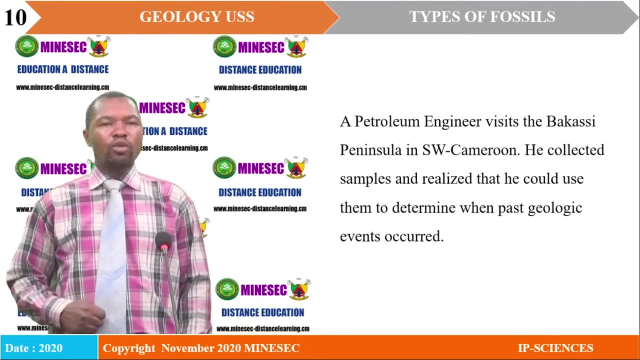 type in both sections. now, this is a scenario that was passing through the mind of a petroleum engineer. so a petroleum engineer visits the Bacassi Peninsula in southwest region of Cameroon. he collected samples and realized that he could use them to determine when past geological events would occur. 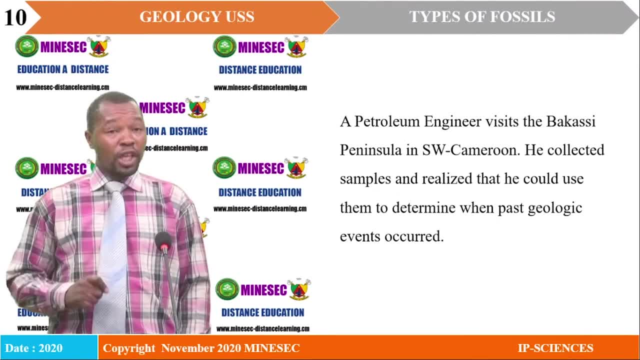 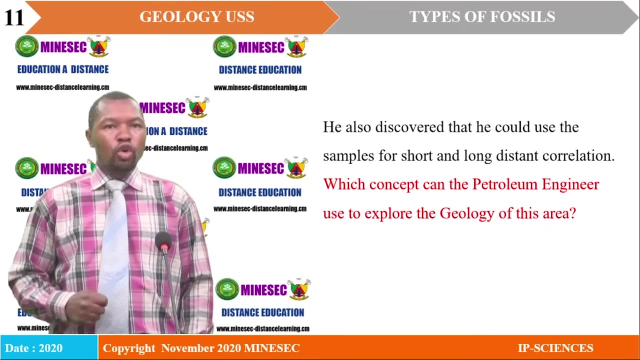 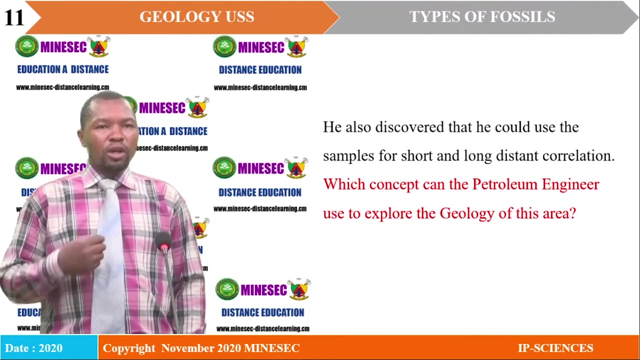 take note. he realized that he could use the samples he collected to determine when past geologic events occurred. now he also discovered that he could use the samples for short and long distance correlation. therefore, which concept can be can the petroleum engineer use to explore the geology of this area? reflect and try to consider some concepts that can assist. 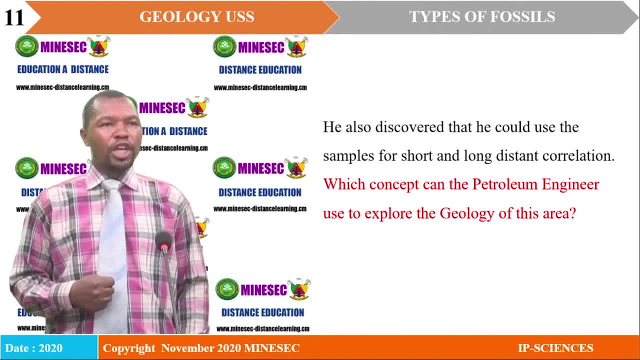 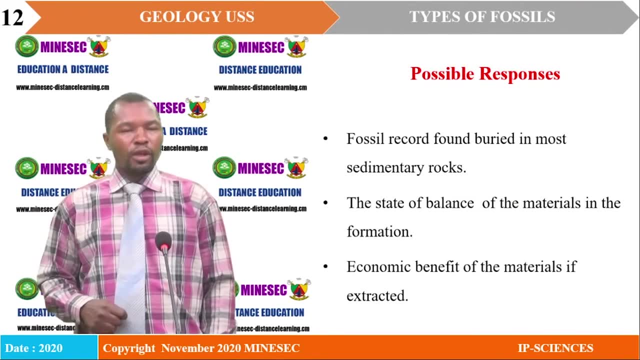 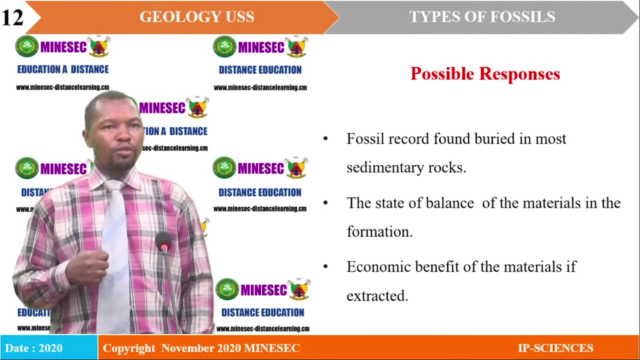 or that can be suitable for the petroleum engineer to explore the geology of this area. The first response: he can use the fossil record found buried within the sedimentary rocks. He can also state: consider the state of balance of the materials in the formation as well. 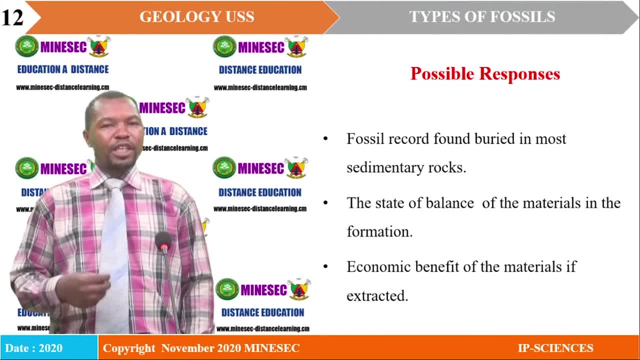 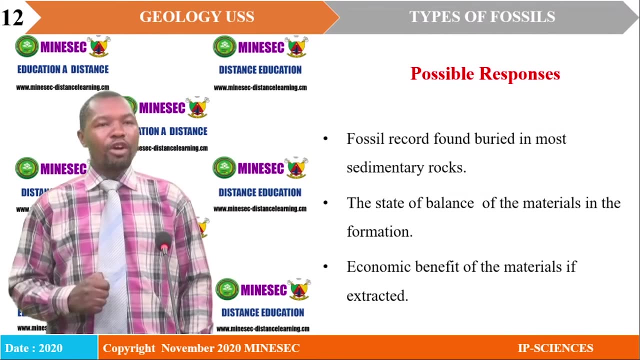 as consider the economic benefits of the materials if they are extracted. Now, in all of these responses, we are going to see which of these responses are the most suitable. They may be correct, but we will see which of them is suitable for the exploration of. 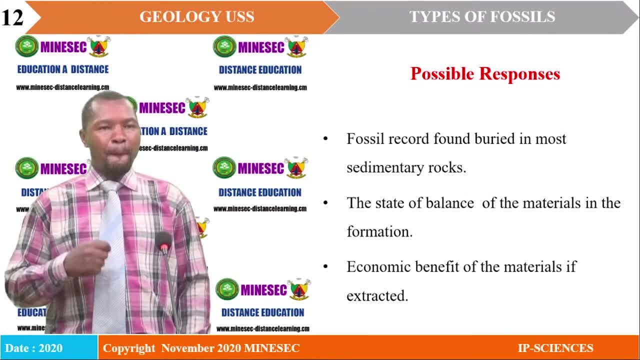 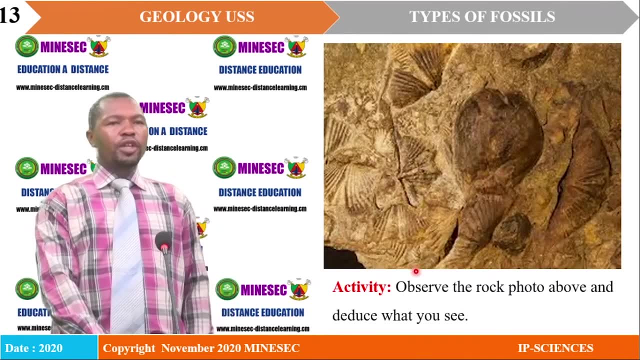 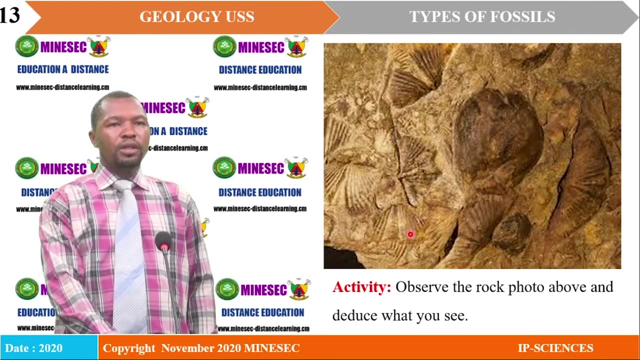 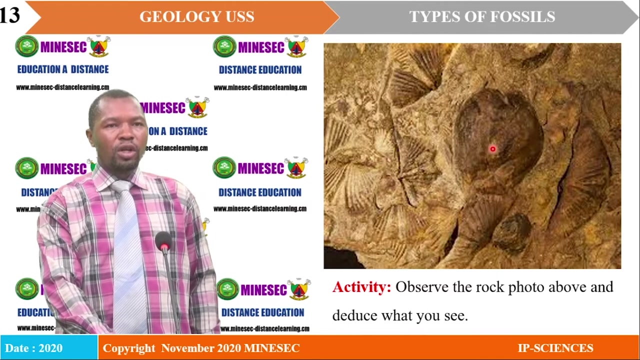 the geology of Bakasi Peninsula. the visit of the petroleum engineer. You observe this photograph and say what you see. You deduce what you see as you look through, Take note of the impressions or these prints or these relics on the rock body. 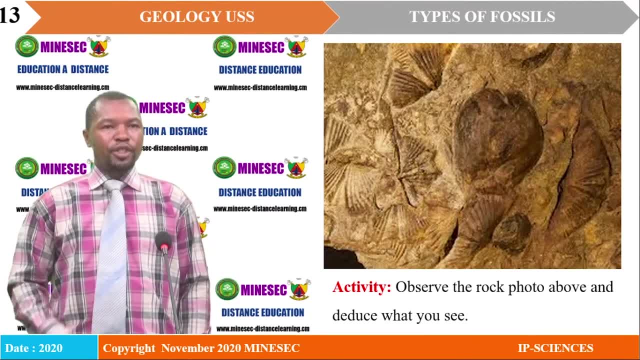 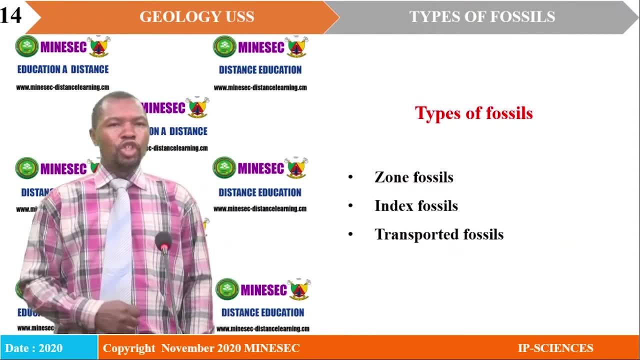 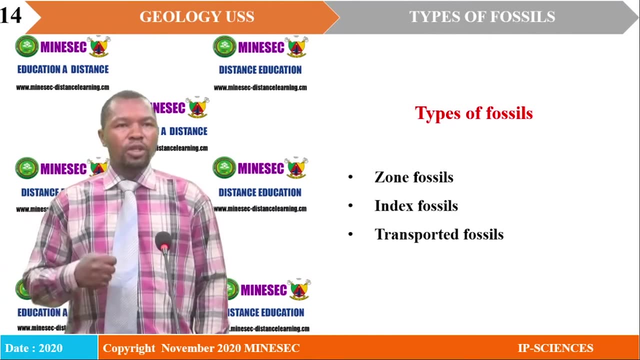 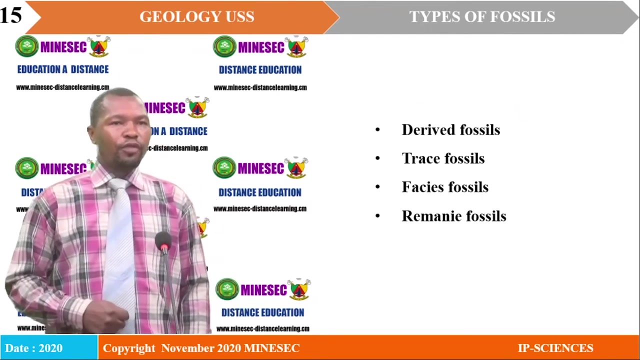 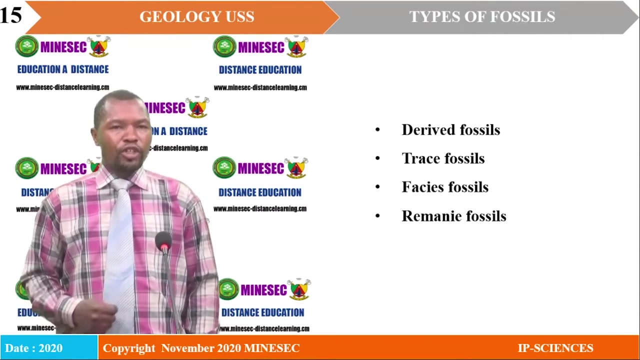 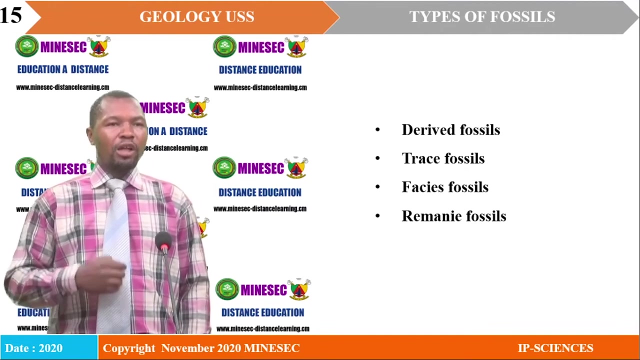 This guides us to the types of fossils. Types of fossils. In geology, there are practically seven main types of fossils. We have zone fossils. Zone fossils Index. fossils Index fossils, Transported fossils. Transported fossils- Tor'". We are going to take each of this fossil type and we shall define them, describe them. 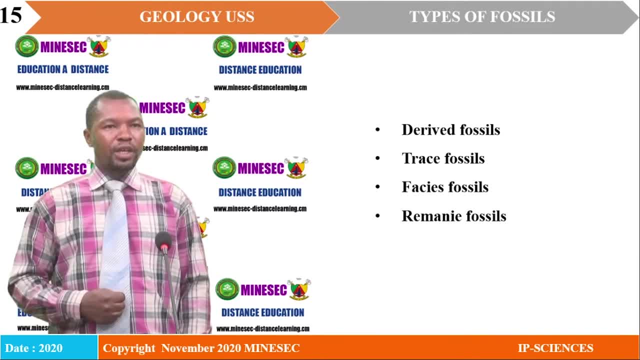 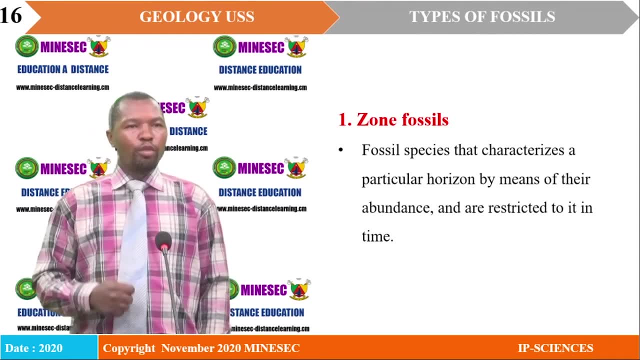 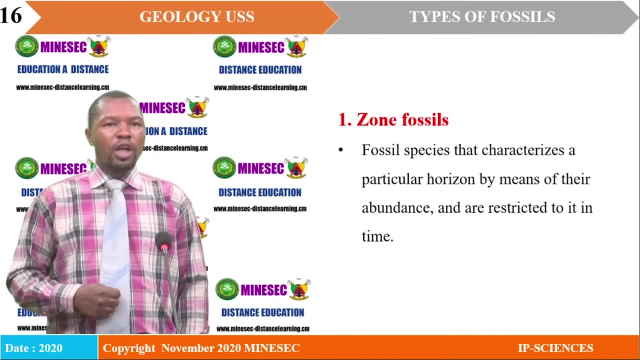 and build up characteristics that are peculiar for each of this fossil type triux. We begin with the first one, that is, zone fossils. Zone fossils are fossil species that characterizes a particular horizon by means of their abundance and are restricted to it in time. 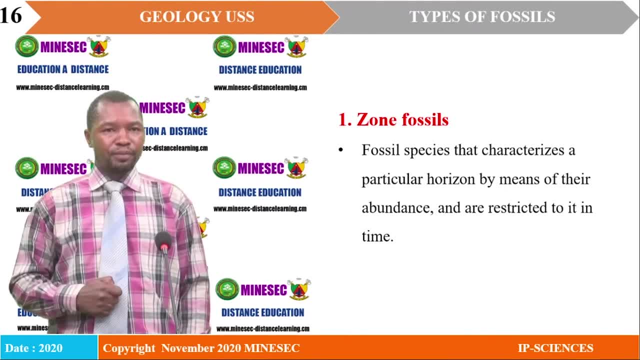 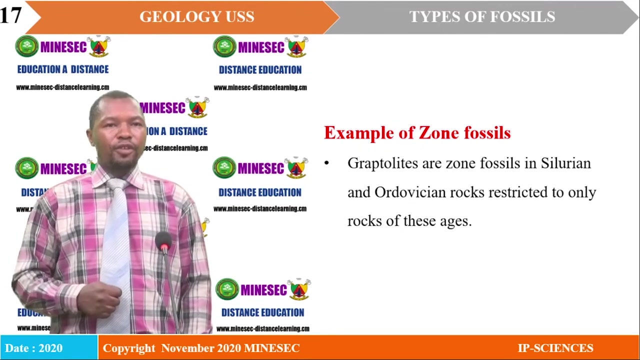 When we talk of time here, we are talking about the geologic time. Remember that the key characteristic value for zone fossils is the fact that they are restricted to the formation where they are found in time. Example of zone fossils: We have a fossil like Graptolite, which are zone fossils in Silurian and Odovisian rocks. 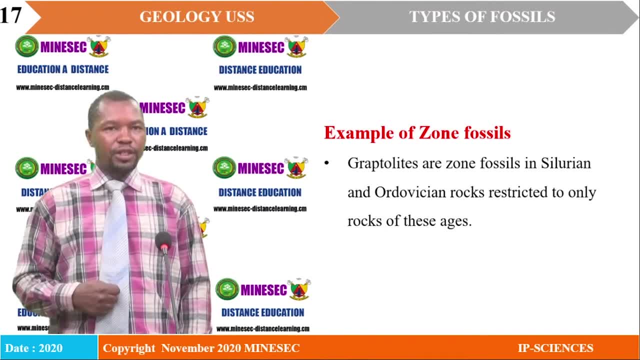 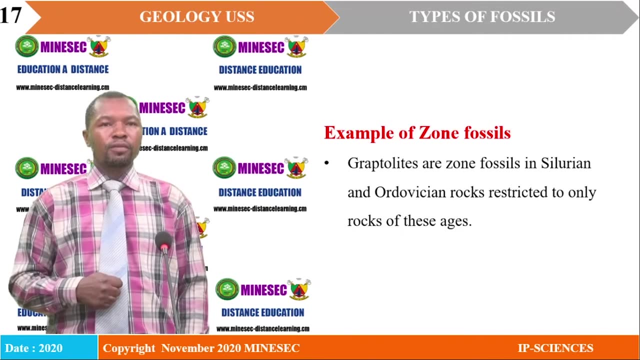 Restricted to only rocks of this ages. Remember that the Silurian and the Odovisian make up the lower Palazzoic in the stratigraphic column which we saw during our lesson four. Therefore, we have these fossils occurring, or Graptolites occurring, shortly after the Cambrian. 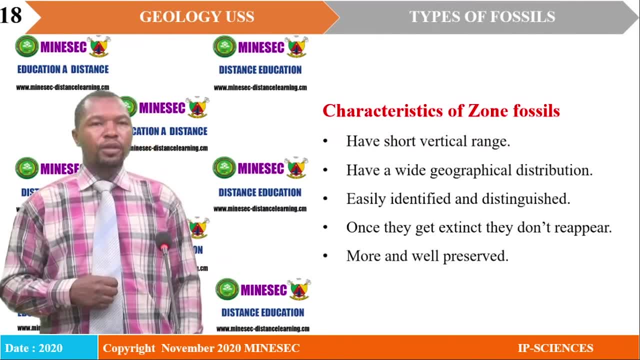 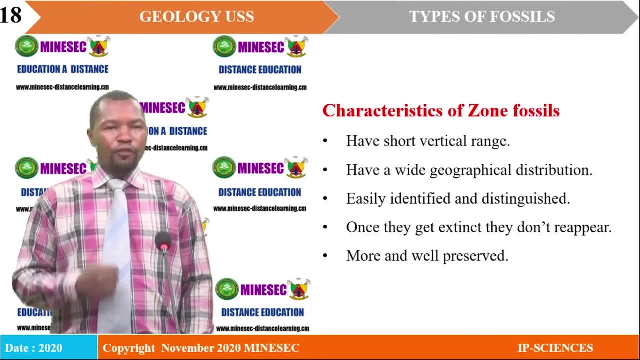 Characteristics of zone fossils. Zone fossils, or, better still, good zone fossils, possess the following characteristics. Number one: they have short vertical range. That means that they have a short lifespan. This group of fossils, again, have a wide geographical distribution. 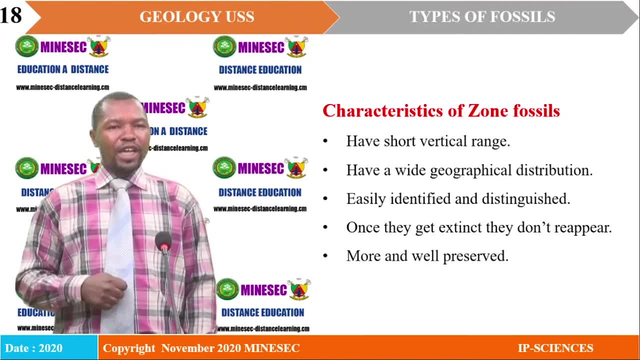 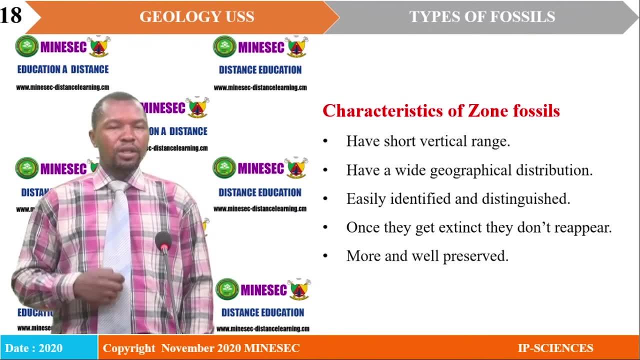 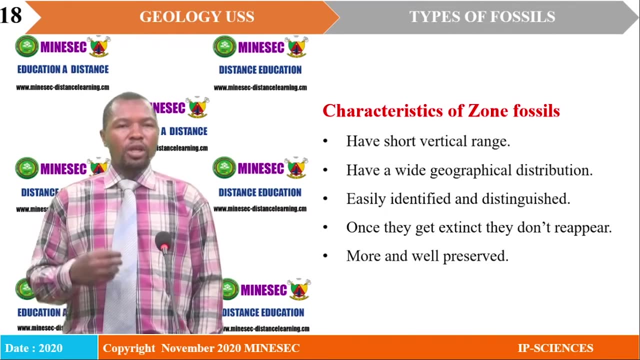 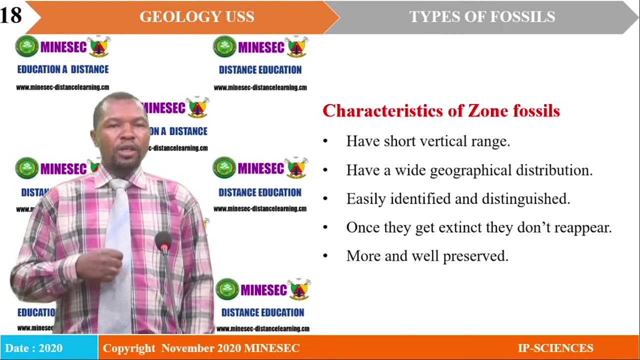 And most importantly, is the fact that they occur In many rock formations found in different localities. This helps them or this guides to the name zone fossils. Also, zone fossils are most easily identified And as well as they are easily distinguished. 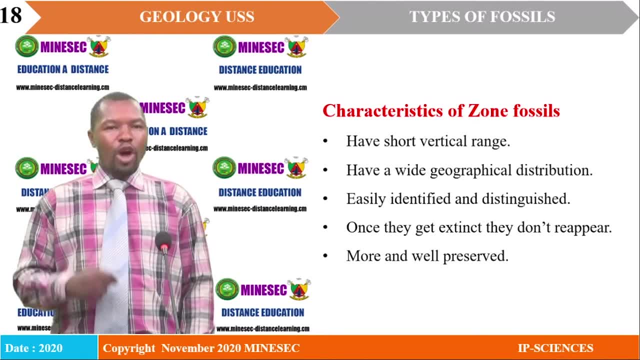 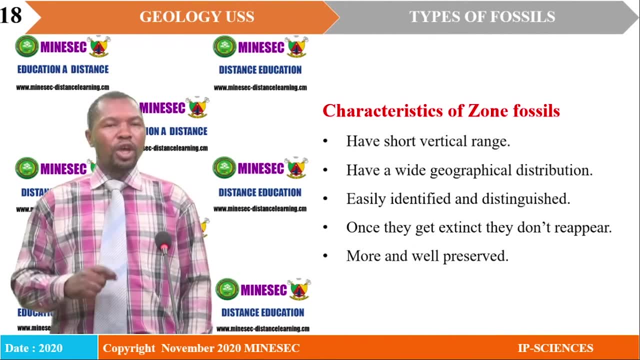 The key thing again is that Once these fossils get extinct, they do not reappear. In other words, we don't have extinct fossils that are supposed to be zone type of fossils, Since they extinct and go at once. We don't have living forms. 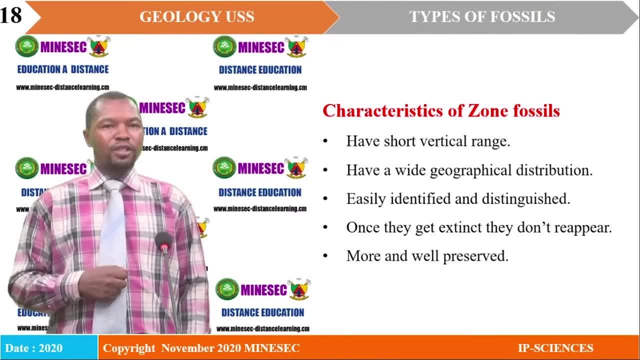 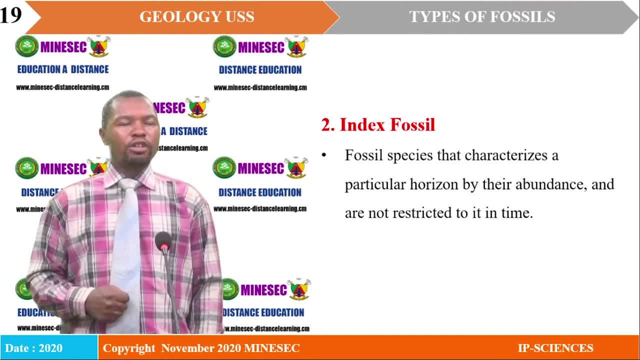 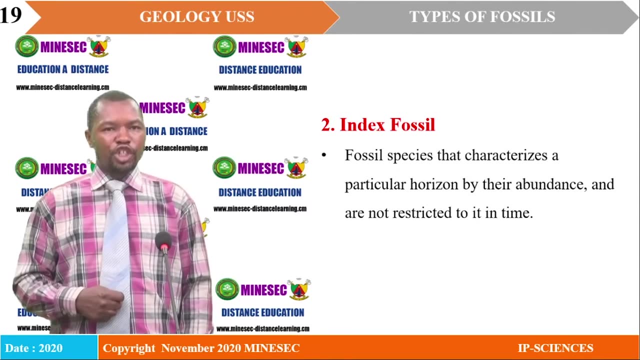 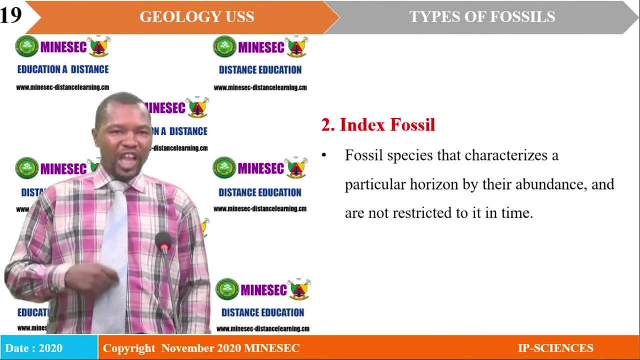 They are more and well preserved. That is one of the characteristics of these fossils. The next fossil type is the index fossil. Index fossils are those fossil species that characterise a particular horizon by their abundance, But this time around they are not restricted to it in time. 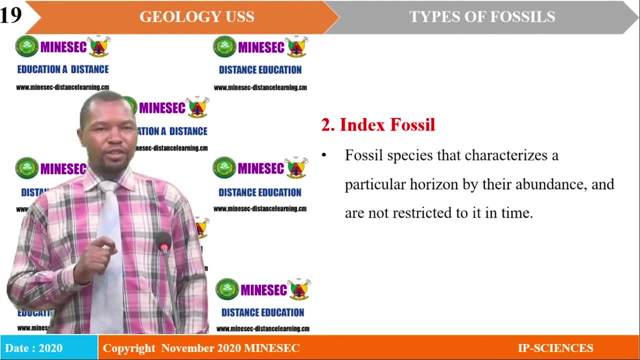 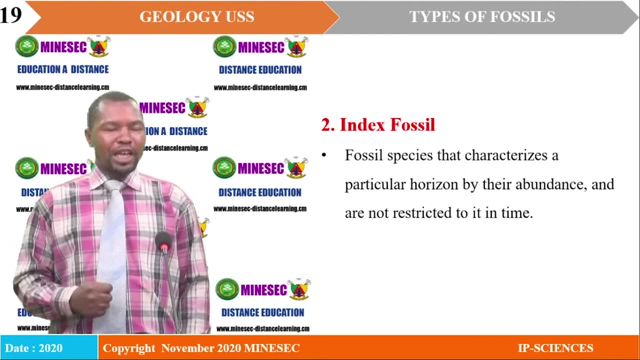 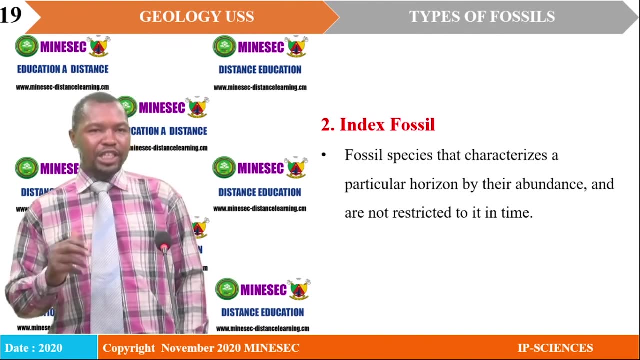 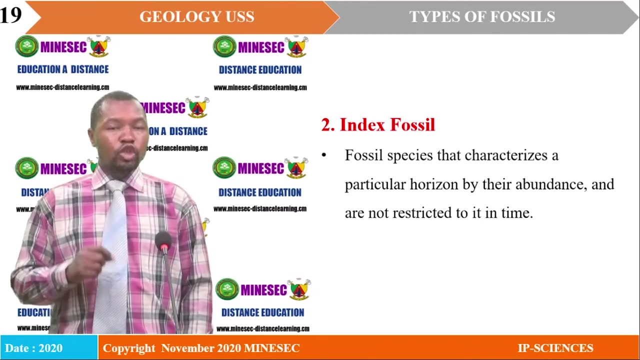 That makes a very thin line difference between index and zone fossils. Remember that, as we saw in our last lessons, the characteristics of both zones and index fossils are very related, but the difference is the fact that index fossils are not restricted to the formation where they find themselves in time. 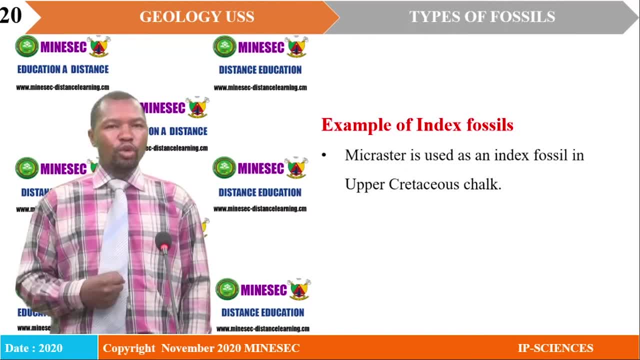 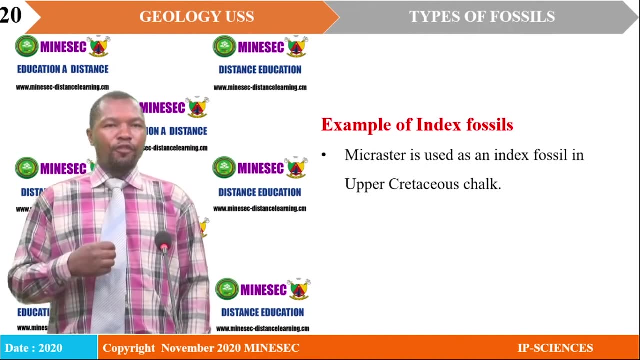 A common example is micraster, which is used as an index fossil in Upper Cretaceous Chalk. The Upper Cretaceous is within the Mesozoic era and it falls at the upper limit where we would have had already Jurassic and Triassic. 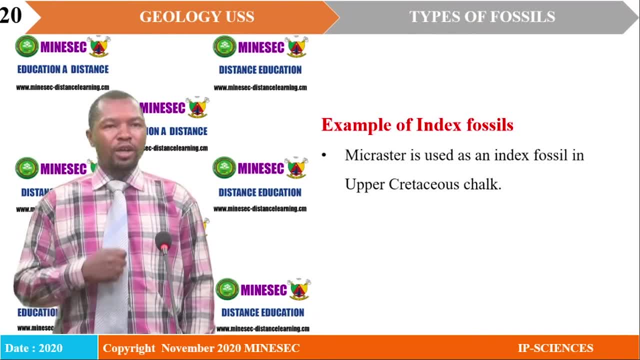 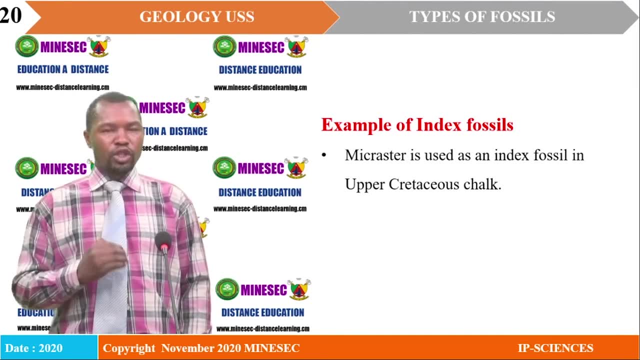 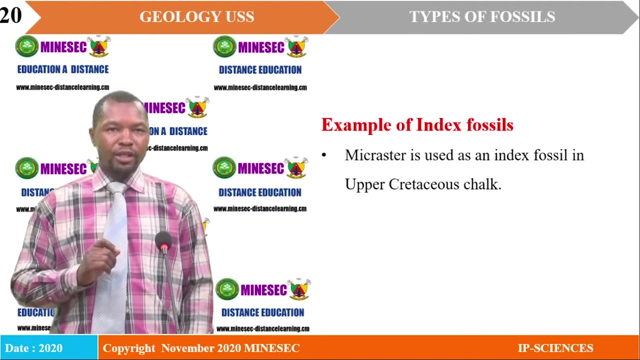 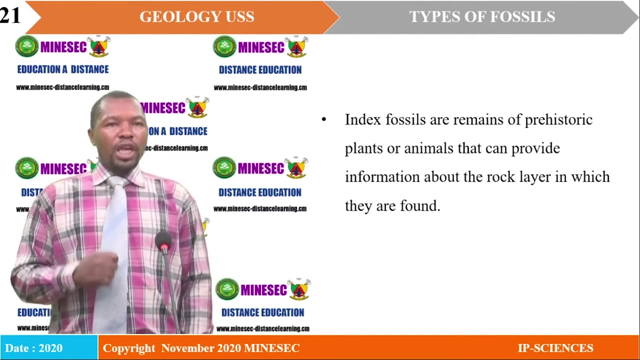 Then we have Lower Cretaceous before the Upper Cretaceous. They make their own, They are indexed to that specifically, If you look at the difference again between the two, with zone fossils we did mention the Silurian and the Odovisian- but with index fossils we are peculiar to the Upper Cretaceous. 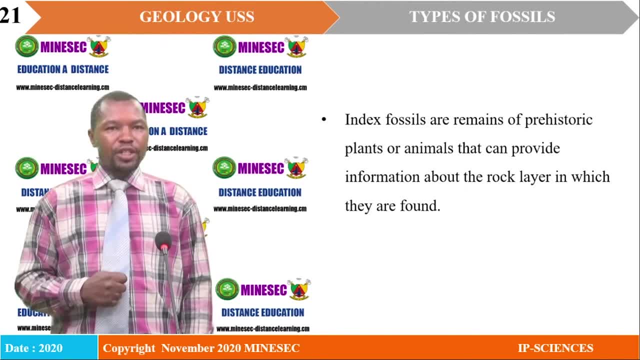 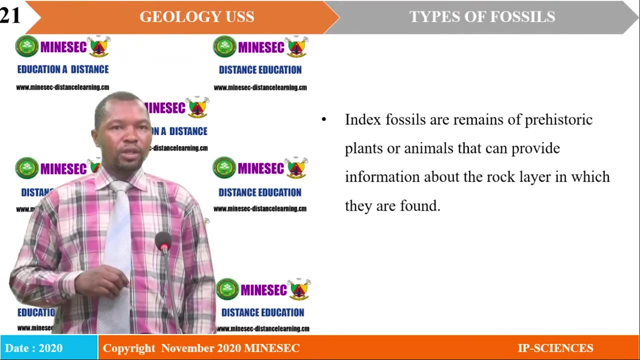 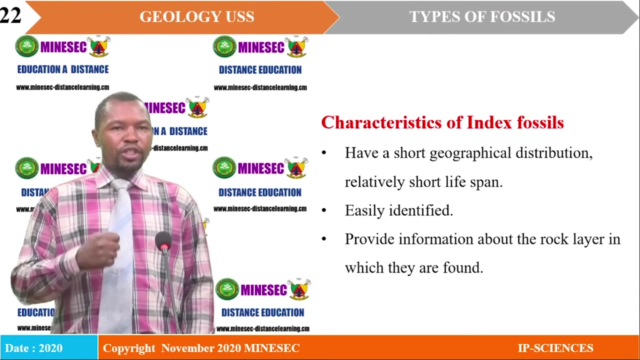 Index. fossils are remains or traces of prehistoric plants or animals that can provide information about the rock We see on random traces of rocks that they are found on that domestic Parce or, as seen on the history of modern safe agent is here By definition. they gained more information on the rock layer in which they are found. 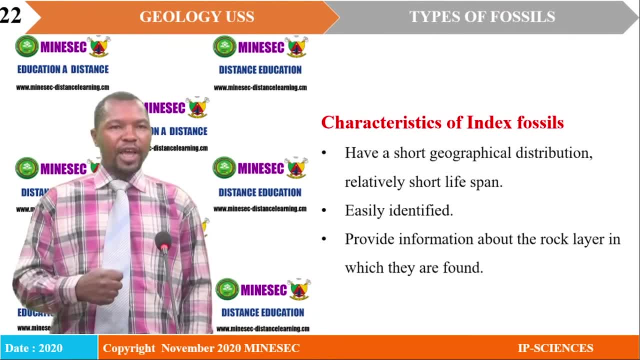 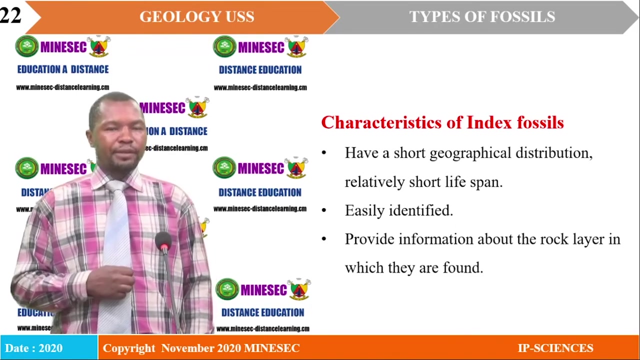 That is very important, The reason for which they are called index, what is called indexed fossils. Indexed fossils all have a short geographical distribution as compared to zone fossils that have a what A wide geographical distribution. That means that these fossil species are relatively- they have a relatively short lifespan. Good, 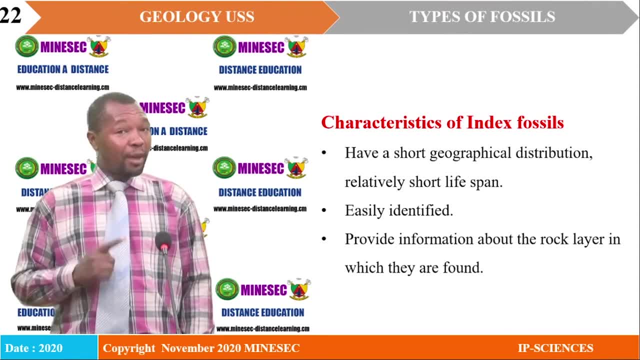 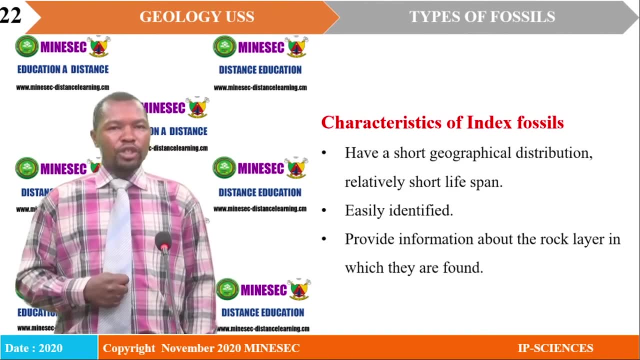 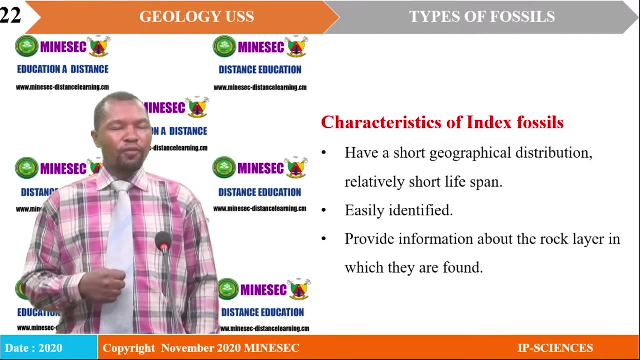 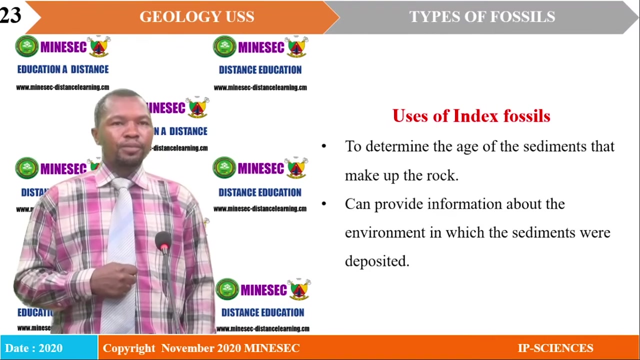 enough is that they are easily identified, but they may not be easily distinguished as compared to zone fossils. They provide information about the rock layer in which they are found. that characterizes indexed fossils. Now, indexed fossils have a wide range of uses as well. These fossils can be used by 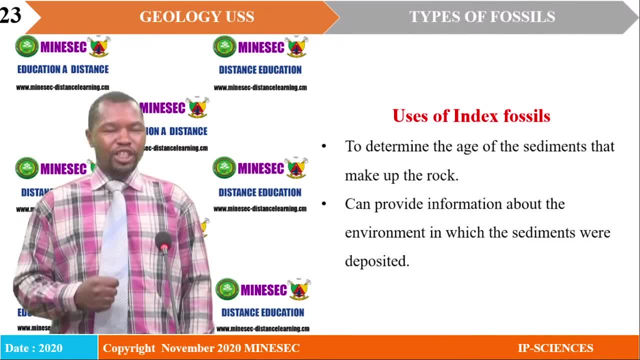 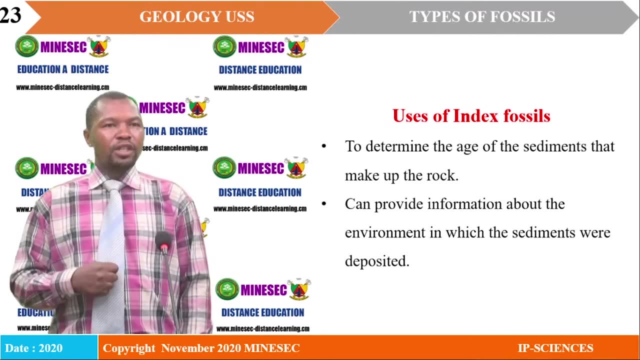 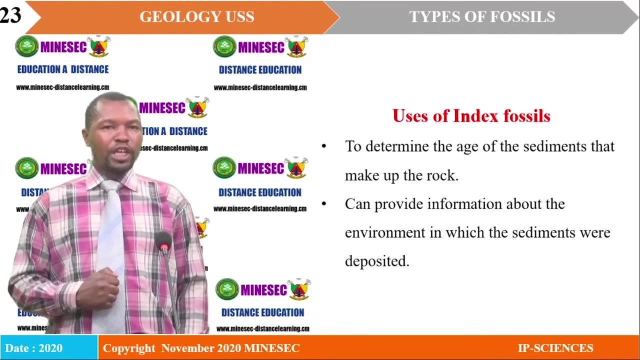 both geological geologists, paleontologists, stratigraphers and petroleum engineers to determine the age of the sediments that make up the rock. Remember that they serve as one of the forces that can be used for correlation, as well as they play the role of the criteria, an important criteria. 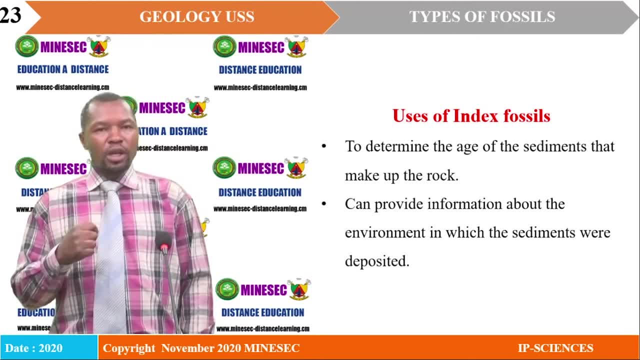 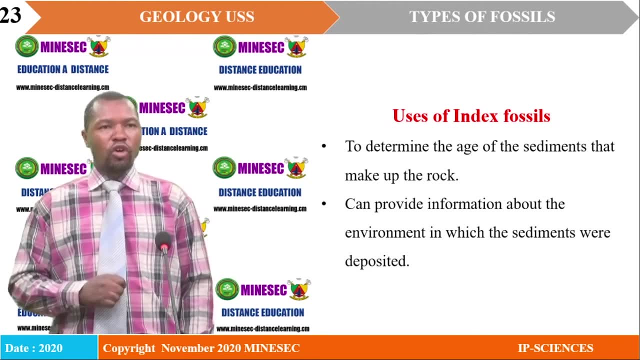 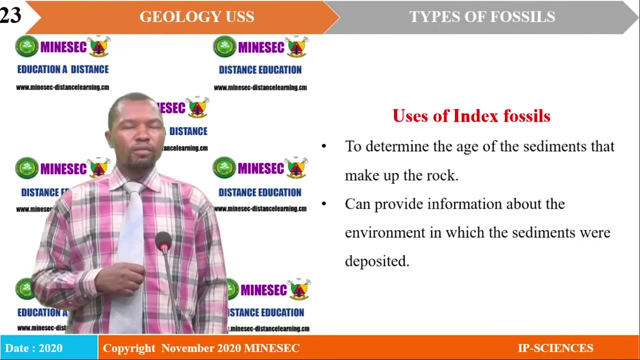 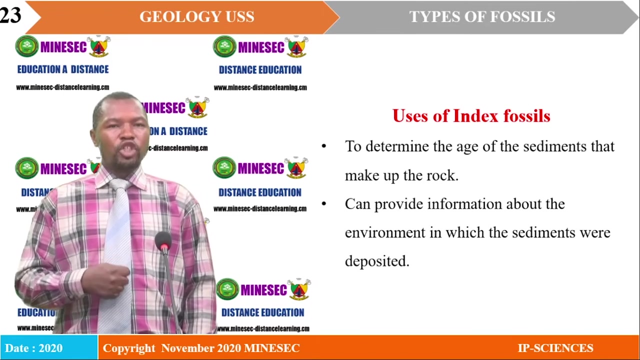 for developing the different divisions of the stratigraphic column which reads the Earth's history and gives us a picture of what geologic events are and at which geologic time they occur. These fossils again can provide information about the environment in which the sediments were deposited. 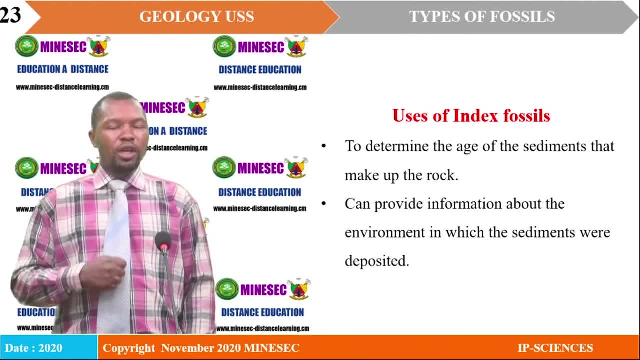 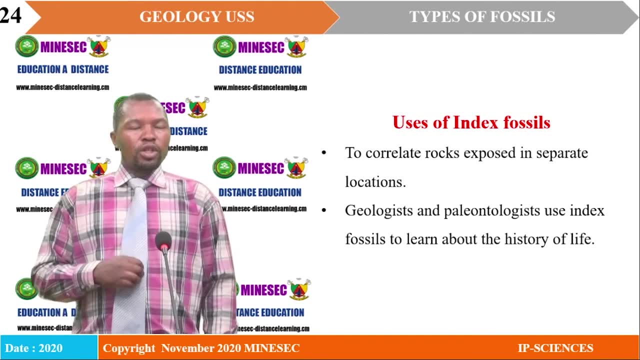 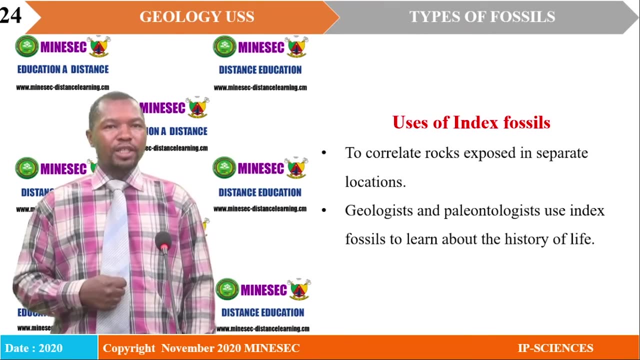 It means that they give us paleoenvironmental information. In other words, they are paleoenvironmental indicators, Zone index. fossils can also be used to compare or to correlate rocks exposed in separate locations. Our lesson, as we saw under stratigraphy, the lesson on correlation of strata: 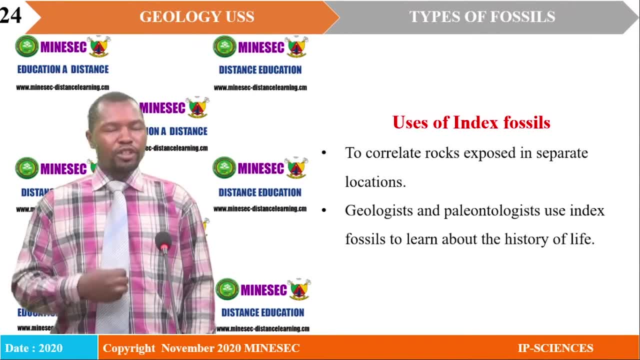 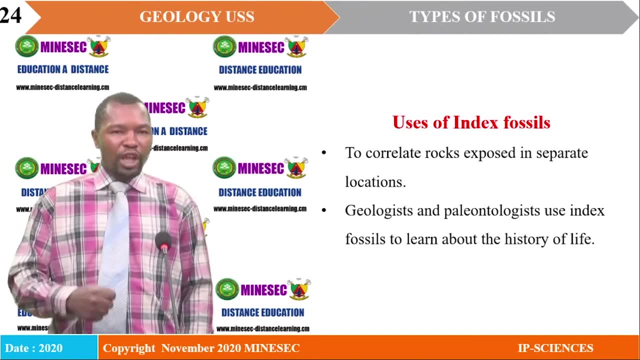 we said that we're looking at fossils that can be used for correlation, and zone fossils, as well as index fossils, were one of them. We want to re-emphasize the fact that in the geologic world, and in the field of paleontology in particular, 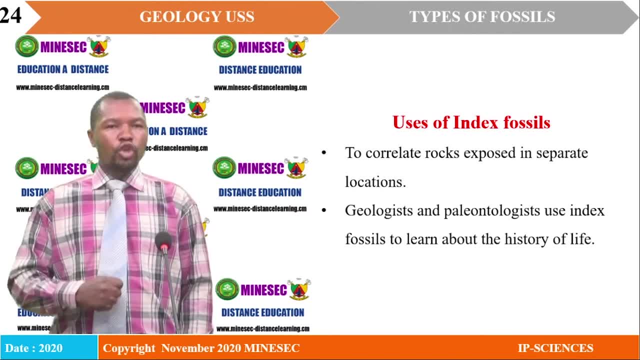 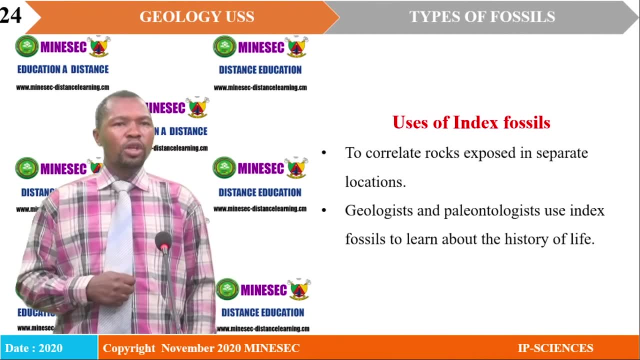 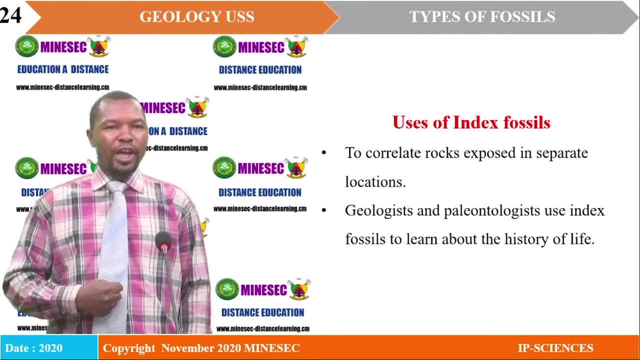 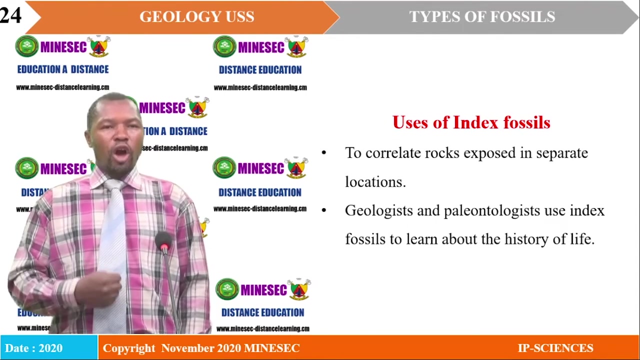 these index fossils will help for us to correlate rocks that are formed in separate localities. Also, geologists and paleontologists use index fossils to learn about the history of the past, the grounds on which the Earth's history has been developed, the grounds to which the age of 4.6 billion years that has been given to the Earth. 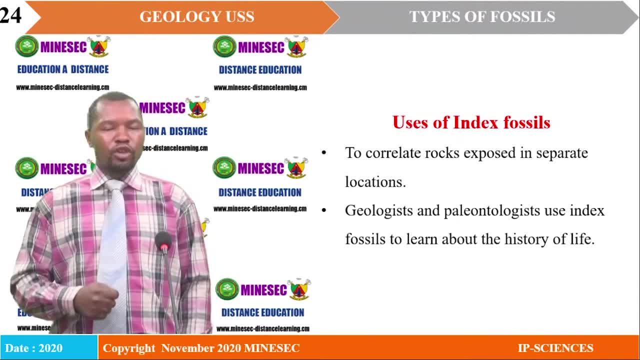 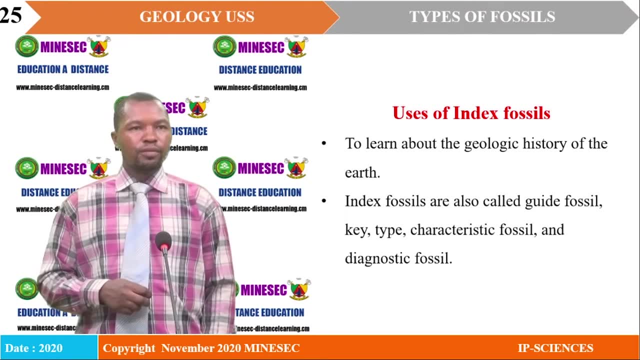 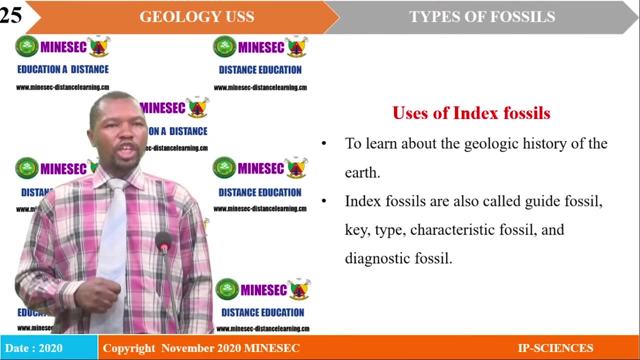 since its origination from the solar system, is developed based on the index fossils Index. fossils, again, are used to learn about the geologic history of the Earth. These are double emphases. They are used. They are used also to be able to give direct information, to give diagnostic information. 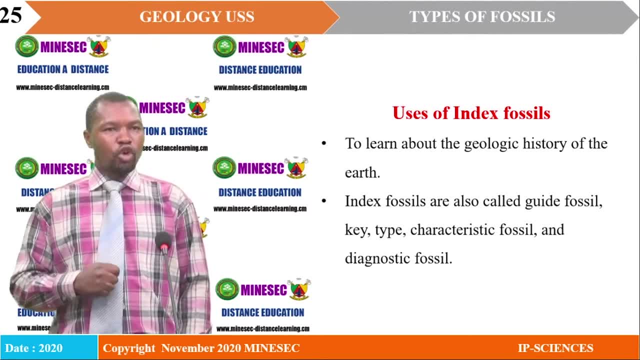 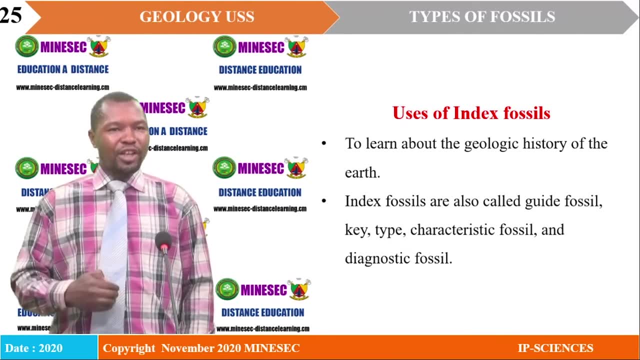 The reason for which we can call them guided fossils or guide fossils. we can also call them key fossils. we can also call them type fossils, as well as characteristic fossils. Then, lastly, we can also call index fossils as diagnostic fossils. 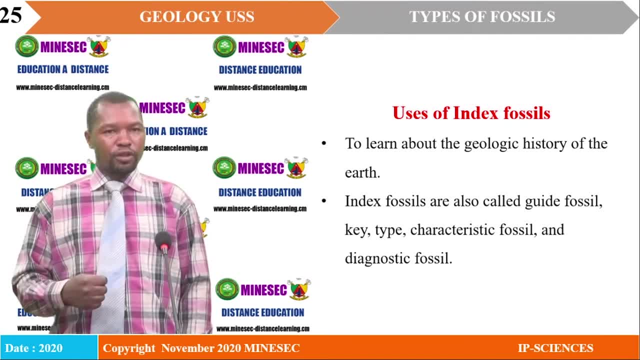 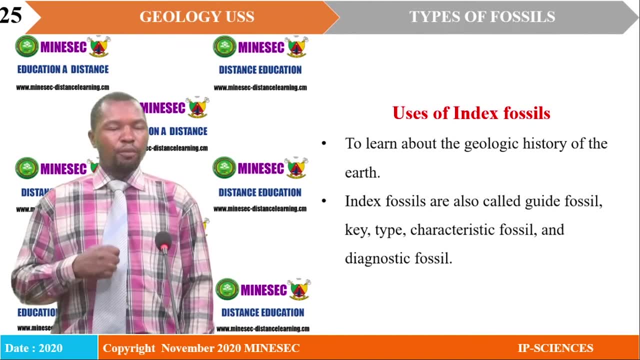 So these are the key uses of index fossils and we want to re-emphasize the fact that sometimes in documents or in information, be it in the classroom, you can see a document pointing a finger at guided fossils, key fossils, type fossils, characteristic fossils, diagnostic fossils. 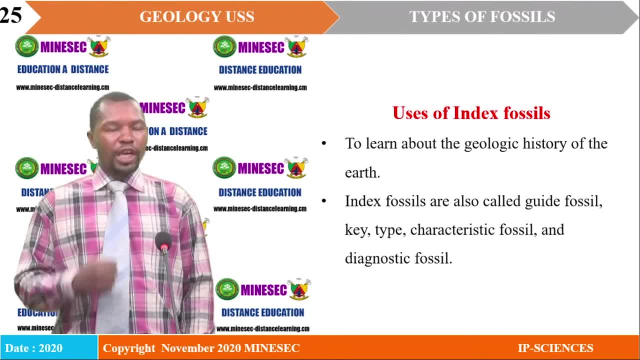 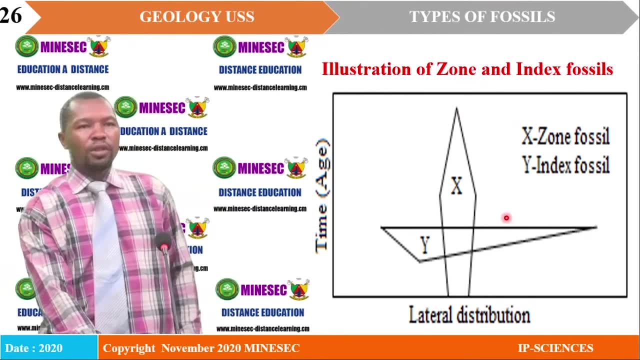 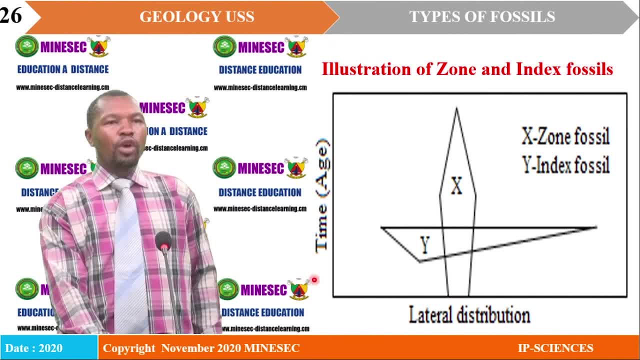 We have this diagram for zone and index fossils From the characteristics that we have seen. we have on the X. on the Y-axis, we have the time, which is H. That is geologic H. Remember that we kept saying that they have a either. 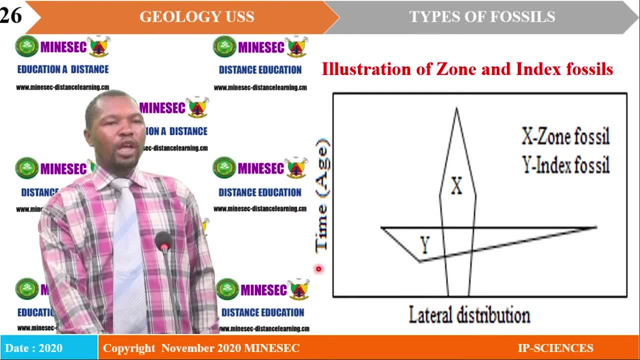 a short lifespan or a long lifespan. We are referring to geologic time, which is the X, the Y-axis, and then we have lateral distribution, which is geographic distribution. If you look at the graph, you will realize that fossil group X is having a long lifespan because it is increasing towards the time, or the age X. 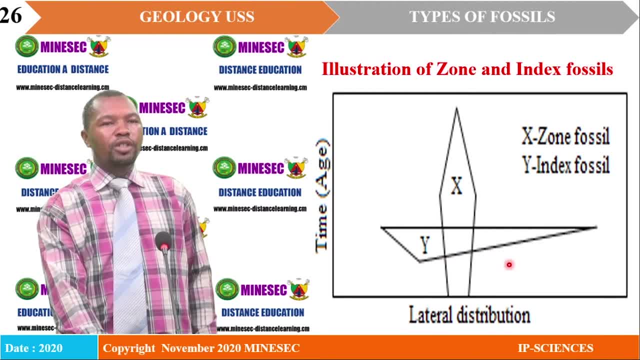 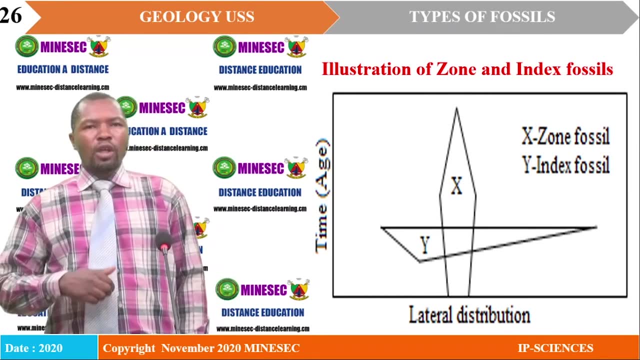 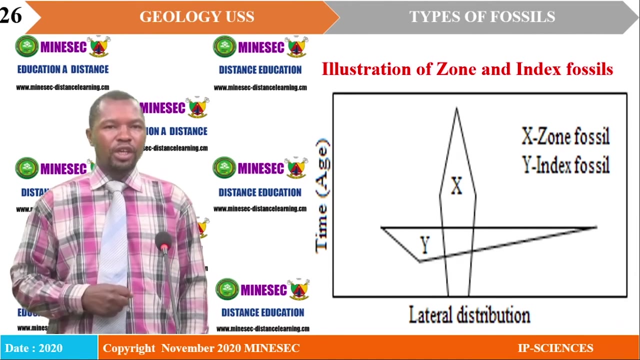 And then the fossil Y is increasing towards the geographic distribution scale or axis, showing that it is widely distributed geographically. So, from the graph, fossil X represents zone fossils, which means that they have a short vertical range, And fossil Y indicates index fossils, which means that they have a relatively short lifespan. 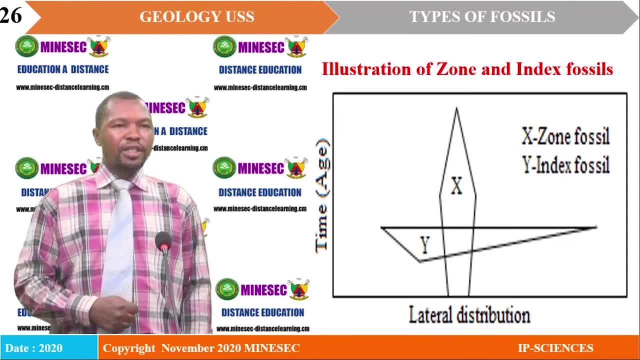 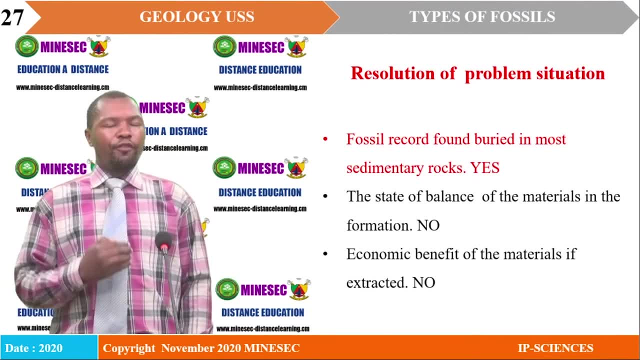 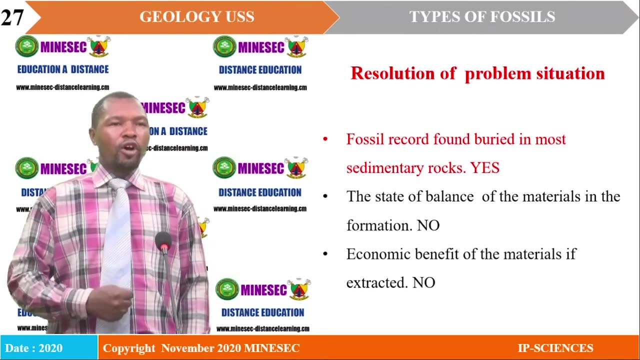 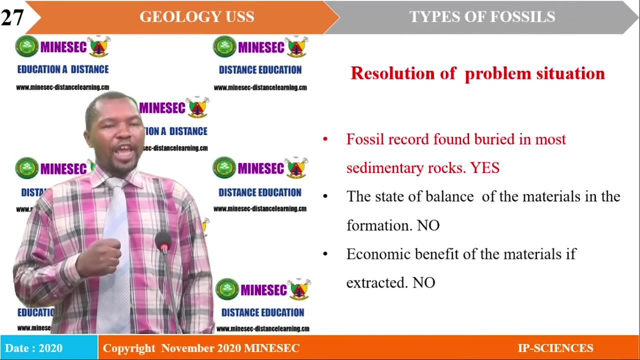 That is the illustration of the index and zone fossils graphically. At the beginning of our lesson we invoked a situation and we're asking ourselves which information is suitable for the petroleum engineer at the Bacassi Peninsula for the exploration of the geology of that area. 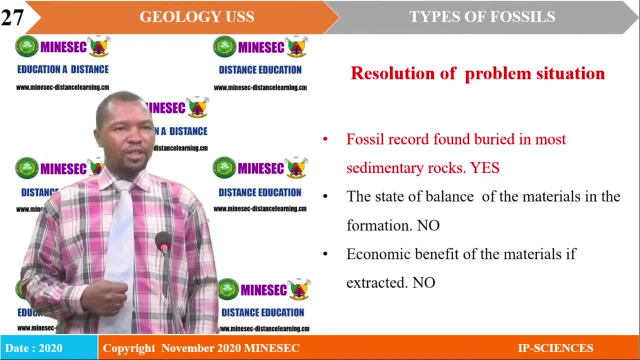 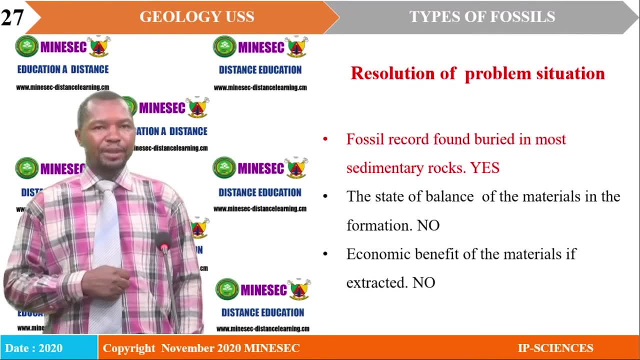 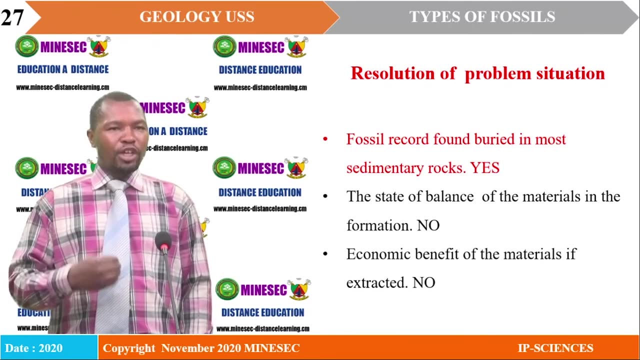 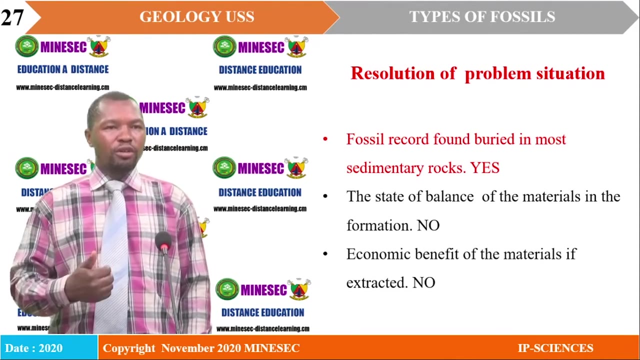 Now we had some responses, the first of which was fossil record found buried in most sedimentary rocks, in the terrain or in that area. Yeah, this From the train of our lesson. we're talking about the different fossil types, meaning that these fossil types can only develop if their records are put in the rocks. 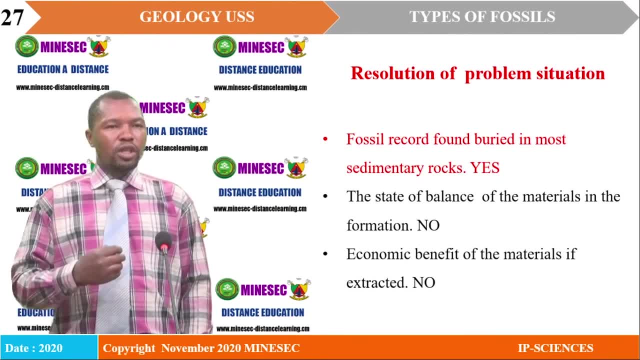 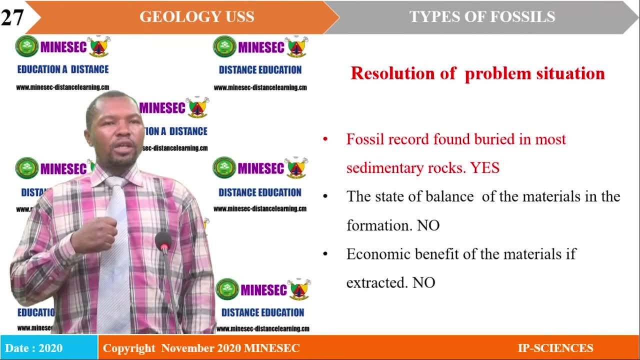 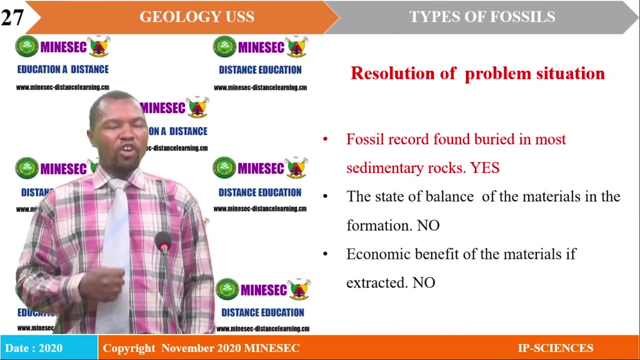 So the first response is acceptable. The second response was the fact that we have to consider the state of balance of the materials in the formation. We said that the state of balance has to do with isostasy. The isostatic adjustment of materials in the area cannot really help us to explore the geology of the area. 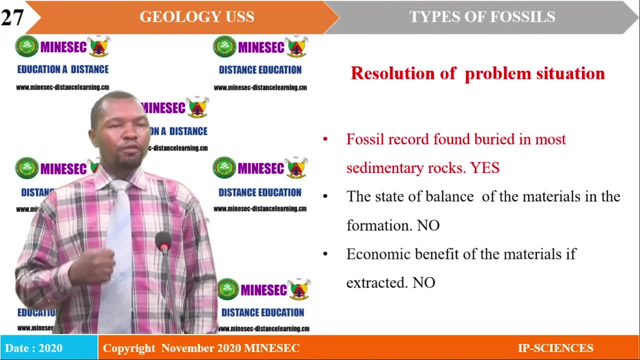 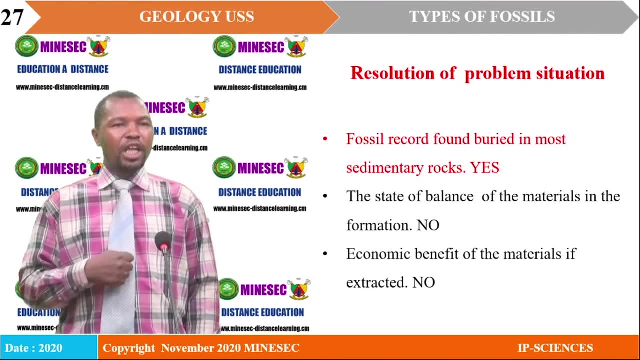 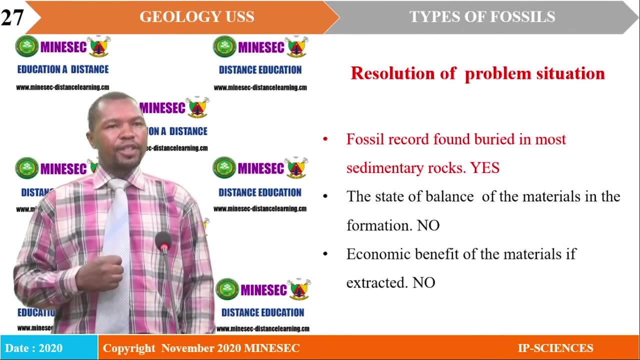 per the information that the petroleum engineer realized that could be useful from the samples collected in the area. Now, the economic benefits of the materials if extracted. Yes, Yes, The economic benefits, But remember that the concern of the petroleum engineer was the fact that he could use it to correlate, as well as develop or determine the age ranges of the materials. 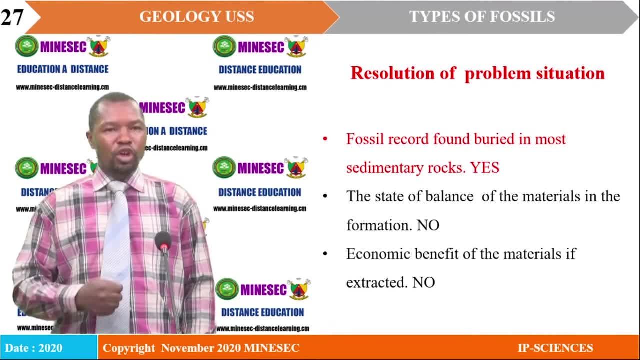 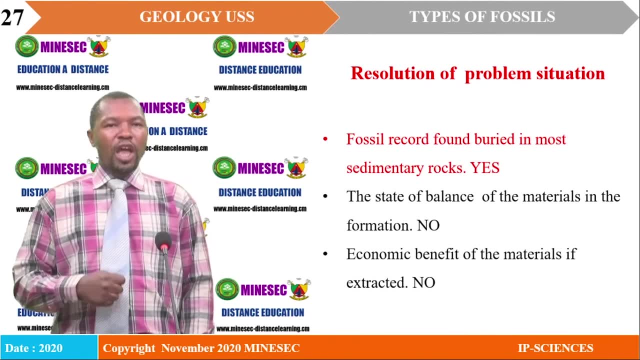 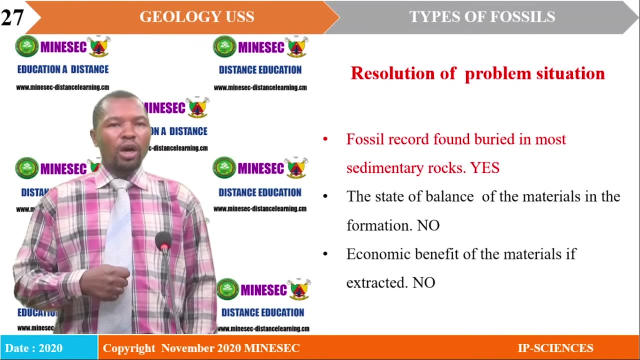 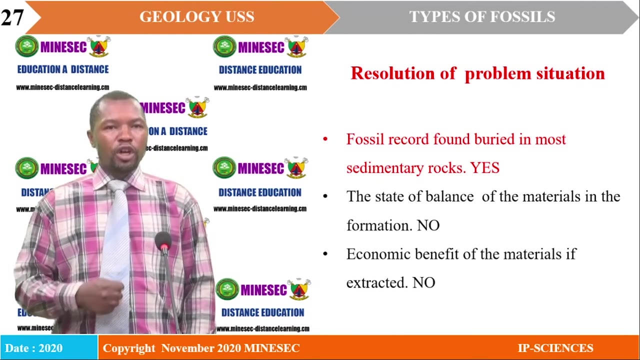 So the last two responses are not acceptable. Therefore, we are saying that the concept that is suitable for the petroleum engineer to explore the geology of this area in which he based on the materials that he collected, should be the fossil record found buried in the sedimentary rocks of the area. 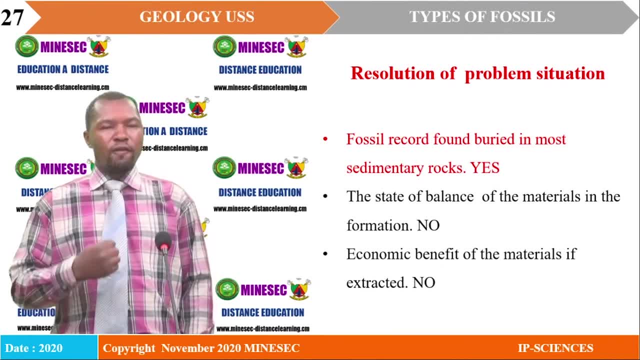 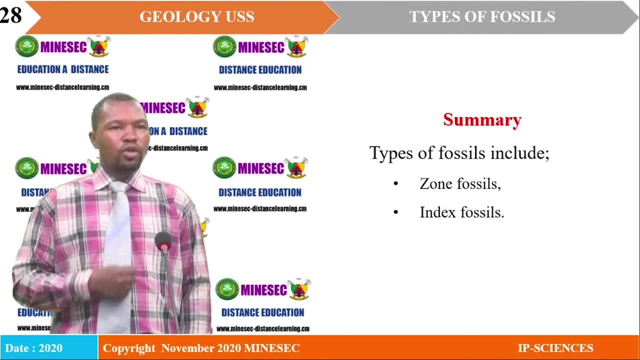 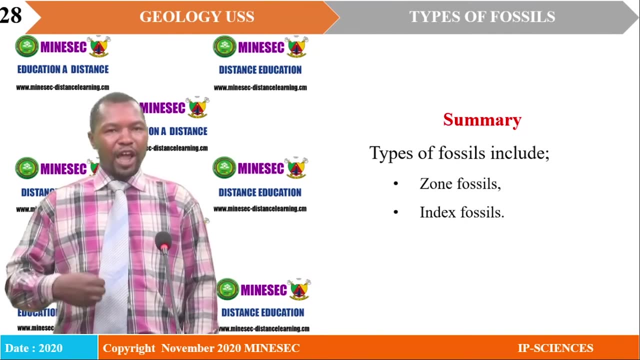 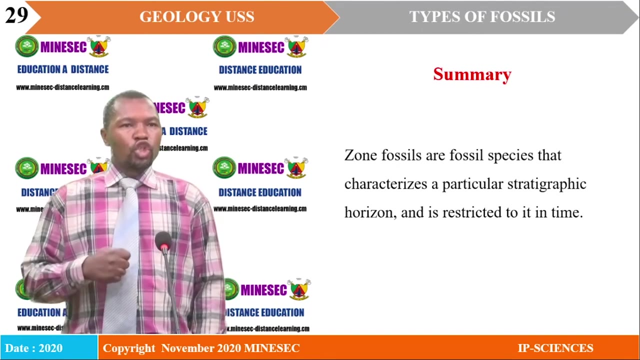 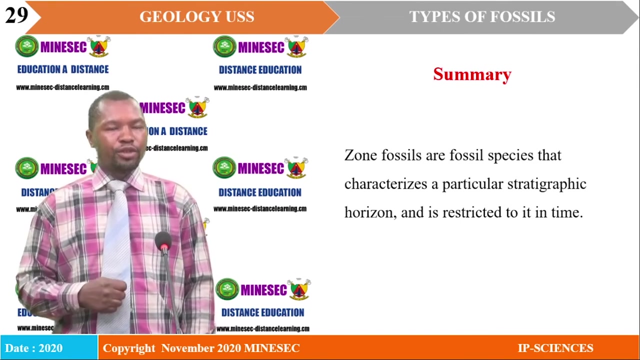 based on our definition of paleontology and fossils. Summarily, types of fossils include zone fossils, index fossils. We have other types, that is, the five others which shall be treated in the next lesson. Zone fossils are fossil species that characterizes a particular stratigraphic horizon and is restricted to it in time. 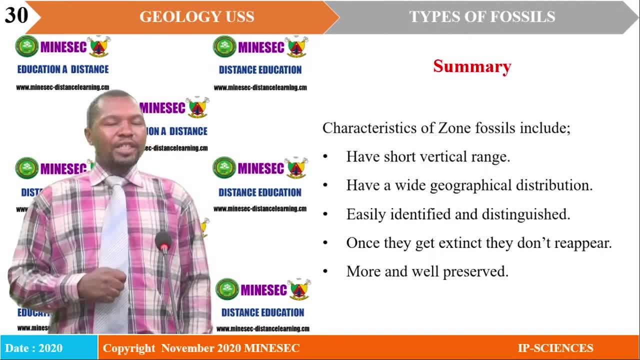 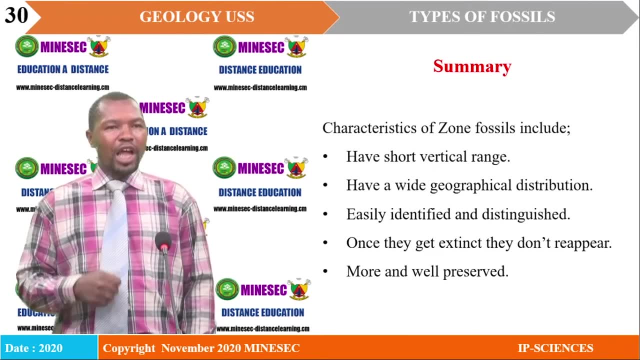 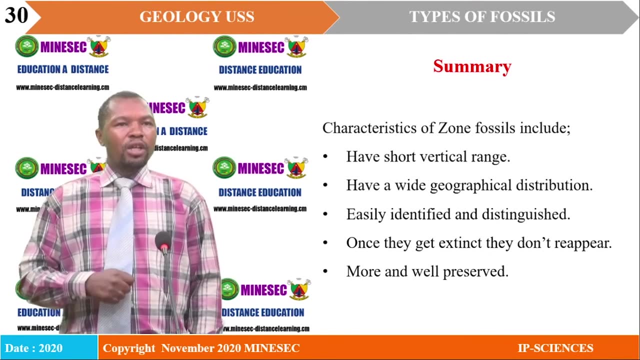 Now, characteristics of zone fossils will include the fact that they have a short vertical horizon, an 600,000 km period of alphabetical range. they have a wide geographic distribution. they are easily identified and distinguished, as well as, once they get extinct, they don't reappear. 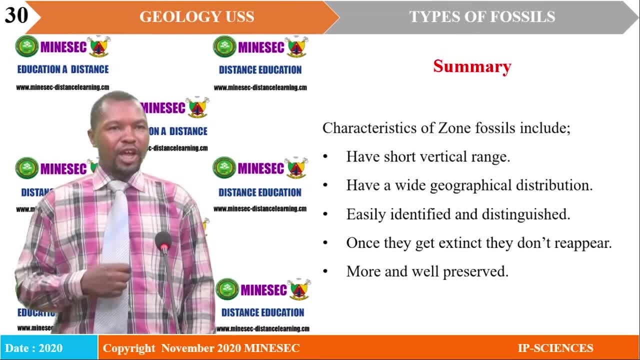 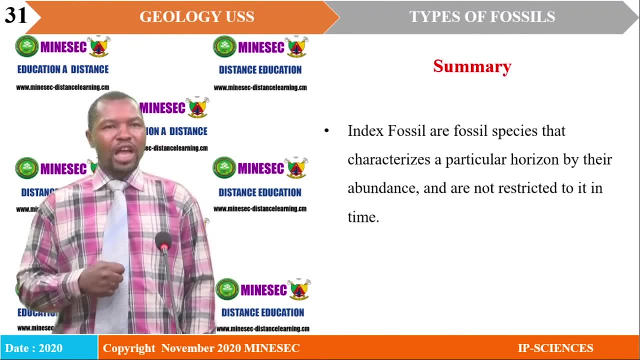 Finally, they are more and better preserved. Indexed fossils are fossil species that characterize a particular horizon by their abundance and are not restricted to it in time. They exist only asash时 and now. They are fine monthly and day ditées. 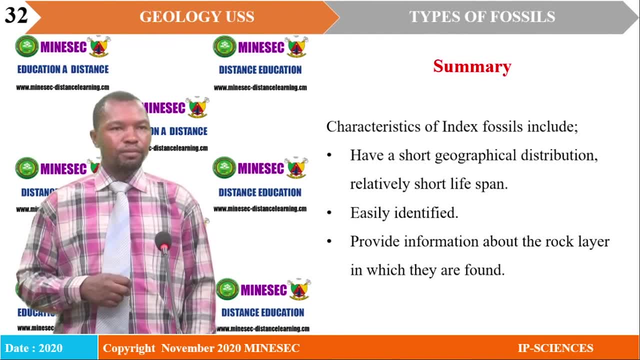 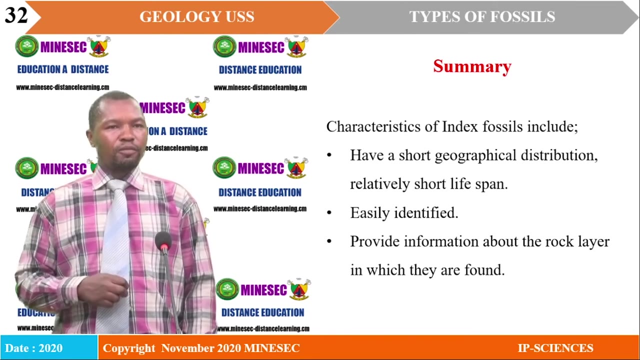 What? until So long, come again. Okay, excuse me to eat in time. Characteristics of index fossils include the fact that they have a short geographical distribution and a relatively short lifespan. They are easily identified. They provide information about the rock layer in which they are formed. Now we are going to look at some activities. 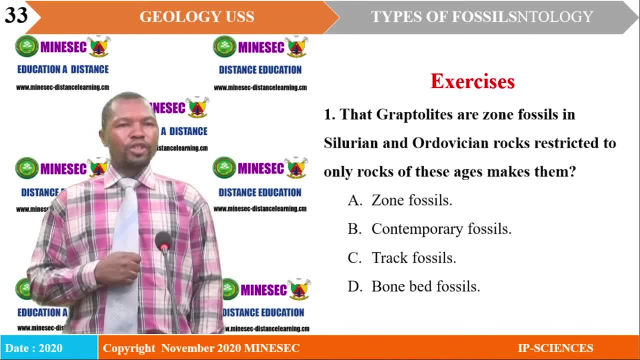 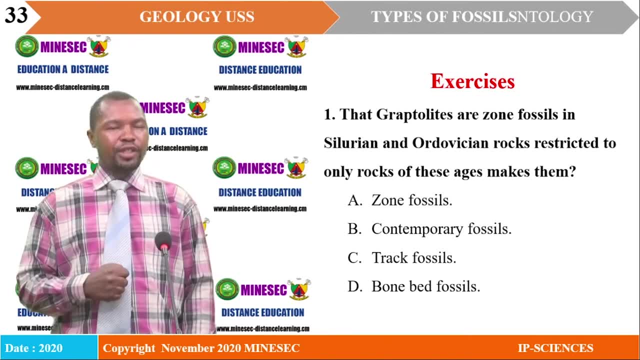 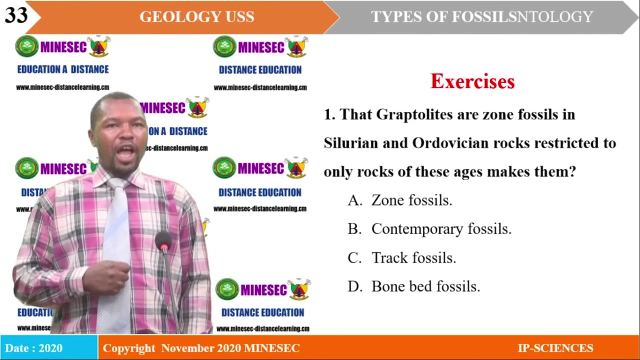 or some exercises, which will help us to better appropriate the lesson, as well as respond to some common elements and key things that characterize our lesson today, which was based on the different types of fossils. Question number one: Vagraptorites are zone fossils in Silurian and Odovisian. 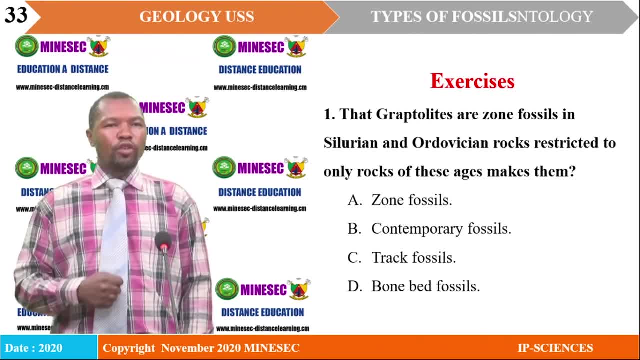 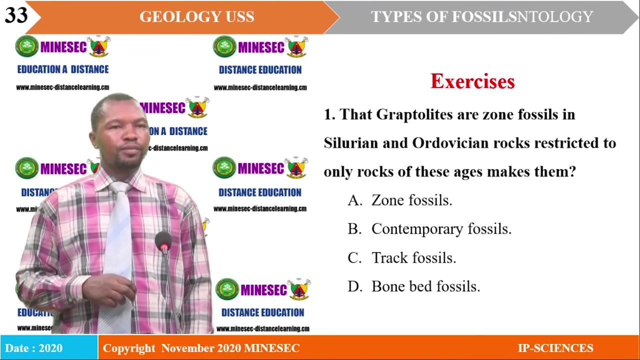 Again that Vagraptorites are zone fossils in Silurian and Odovisian rocks, Restricted to only rocks of this age, makes them: A- Zone fossils, B- Contemporary fossils, C- Track fossils. D- Bone bed fossils. Our correct answer is A. 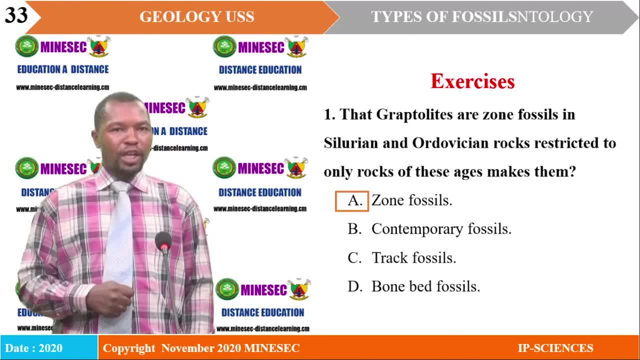 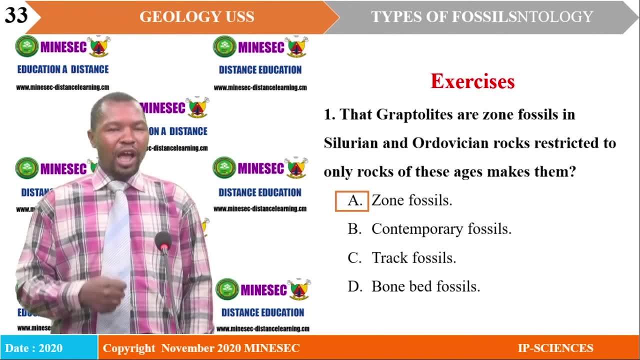 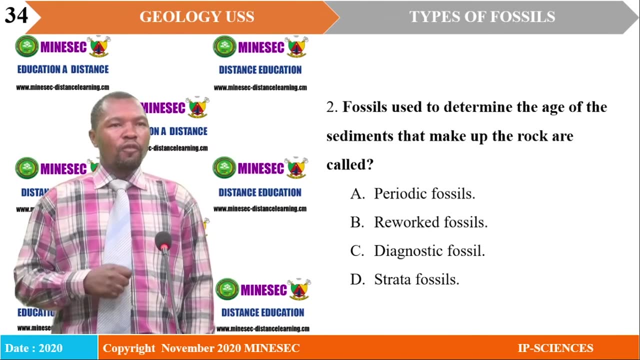 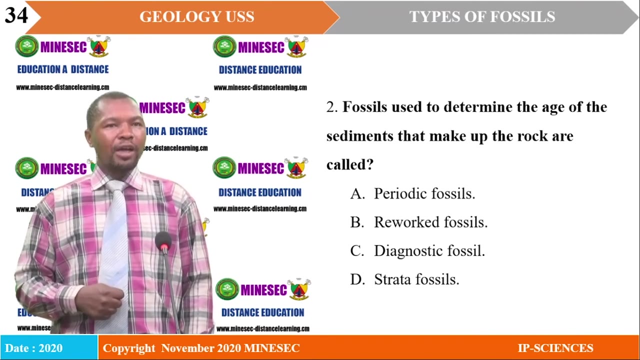 Vagraptorites are zone fossils. Exercise number two: Fossils used to determine the age of sediments that make up the rock are called: A- Periodic fossils, B- Reworked fossils, C- Contemporary fossils, D- Contemporary fossils. D- Bone bed fossils. 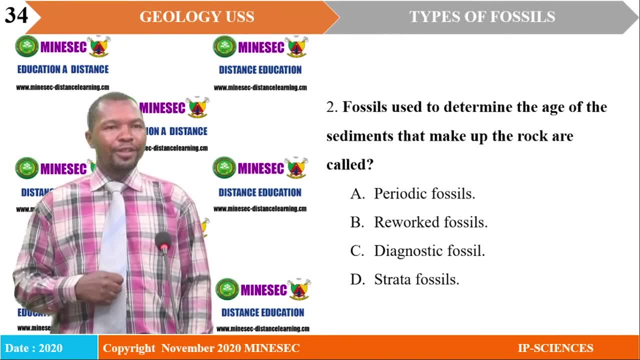 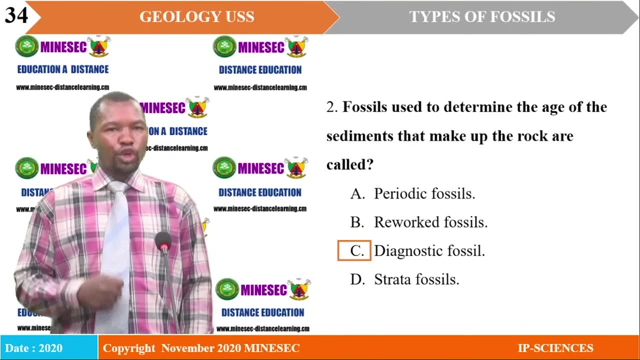 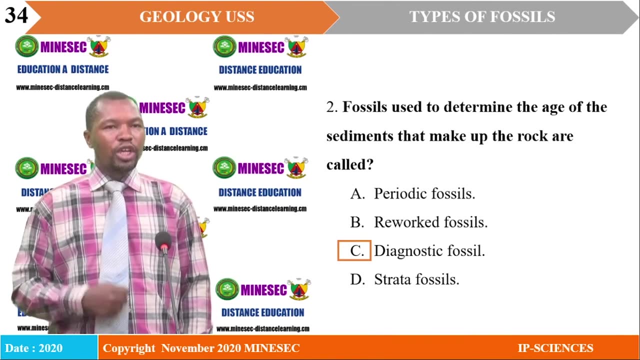 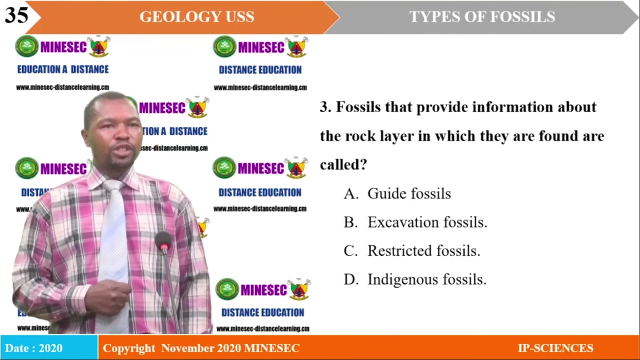 C- Dynostic fossils, D- Strata fossils. Our correct answer is C. Fossils used to determine the age of sediments that make up the rock are called A Dynostic fossils. Exercise number three: Fossils that provide information about the rock layer in which they are found are called 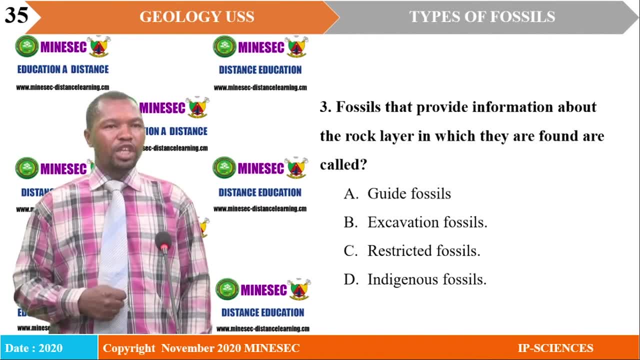 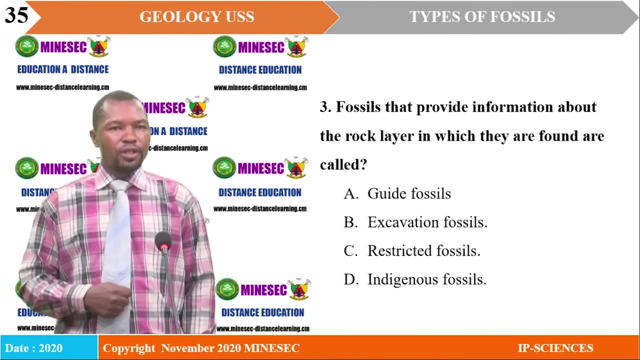 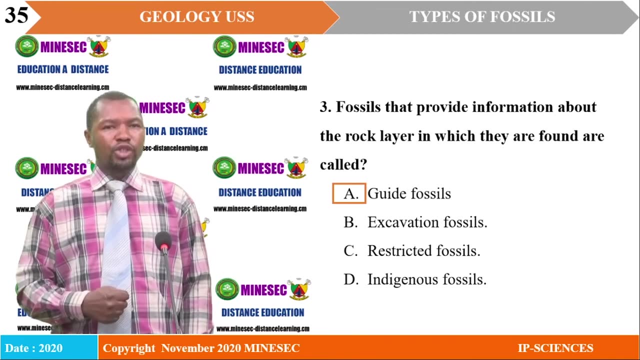 A- Guided fossils or guide fossils. B- Excavation fossils. C- Restricted fossils. D- Indigenous fossils. Our correct answer is A. We are saying that fossils that provide information about the rock layer in which they are found are called guide fossils. 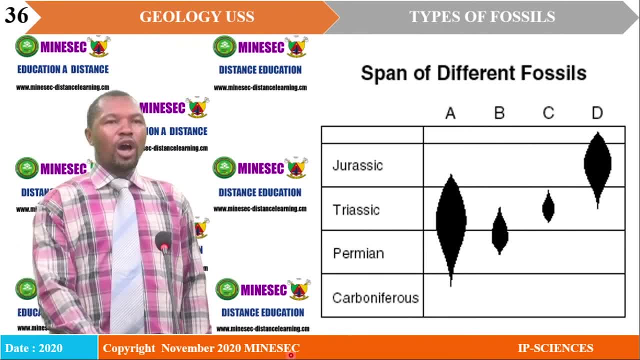 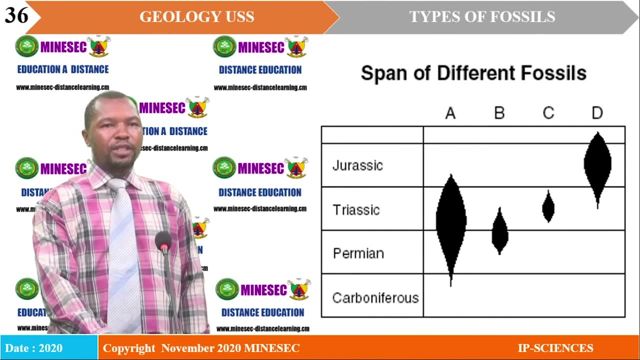 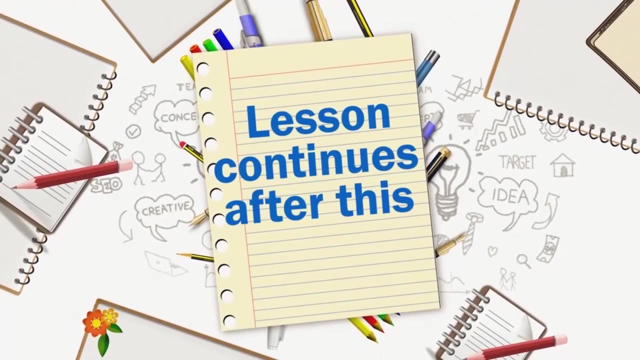 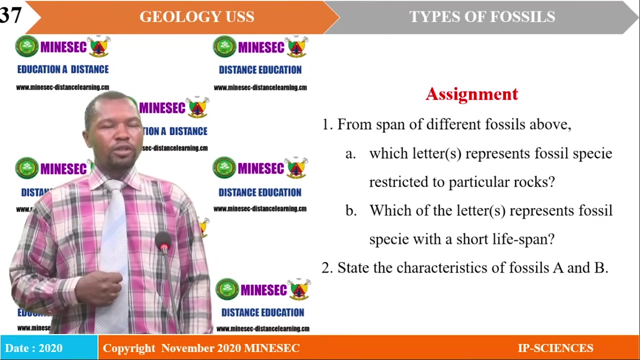 You are going to, at home, work on this diagram. That is the lifespan or span of different fossils. You observe it, Look at the stratigraphic session and how they are represented, And with that at home, you will have to from the lifespan of different fossils that we have just seen. 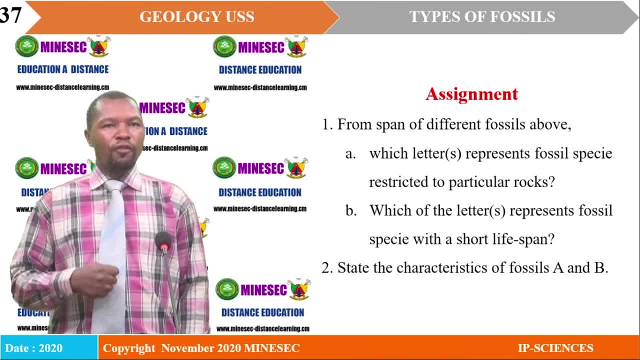 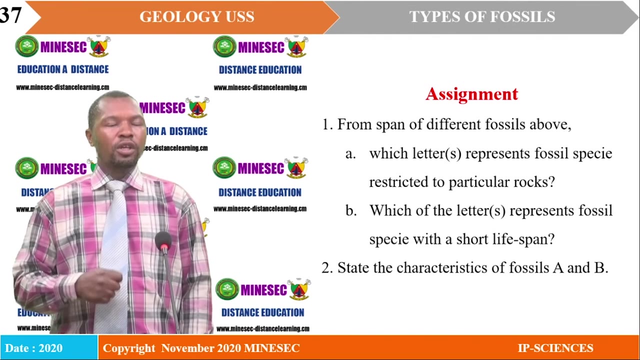 you will say Letters represent fossil species restricted to particular rocks B. You will equally say which of the letters represent fossil species which have a short lifespan. And secondly, you shall state the characteristics of fossils A and B as represented on the span of different fossils. 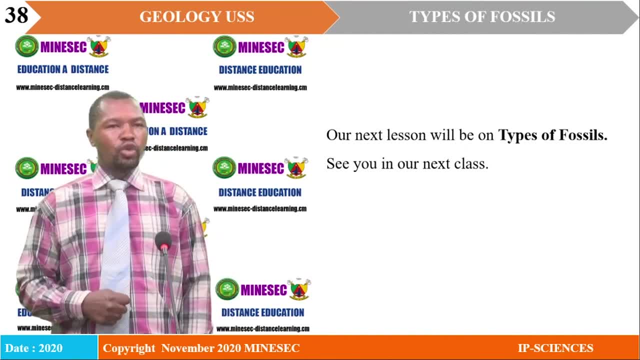 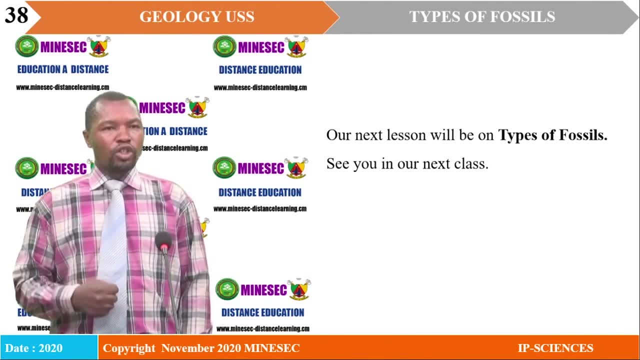 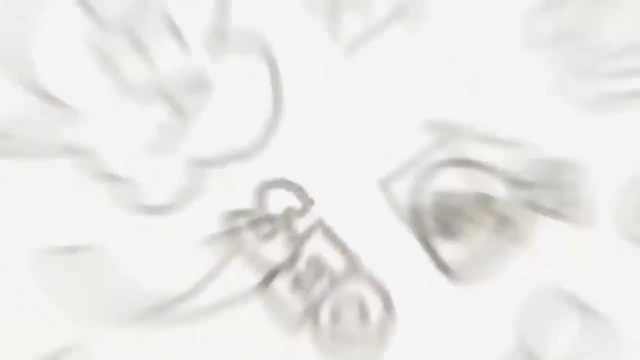 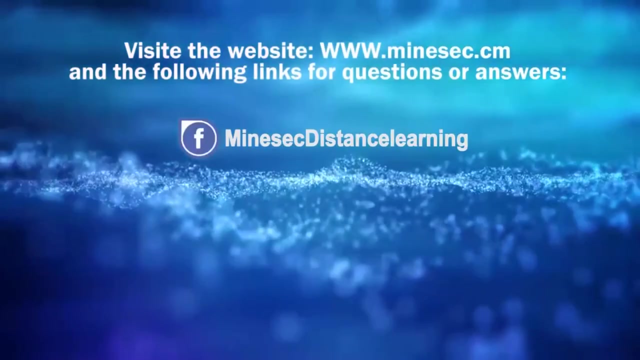 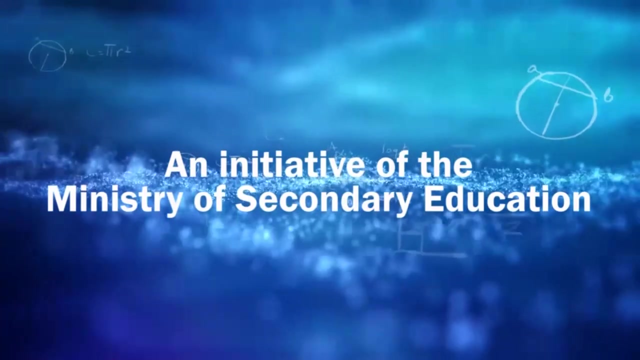 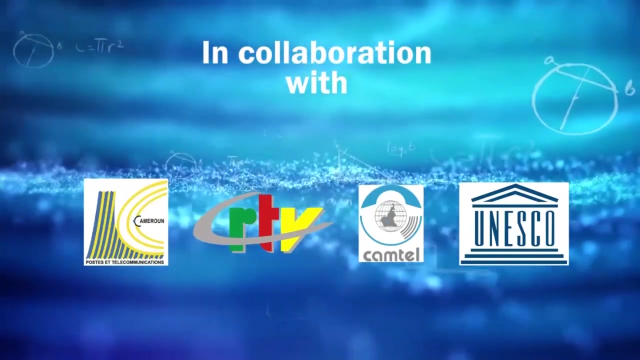 We have come to the end. Our next lesson will be on types of fossils. We will continue to explore the different types of fossils. See you in our next lesson. Transcription by CastingWords.